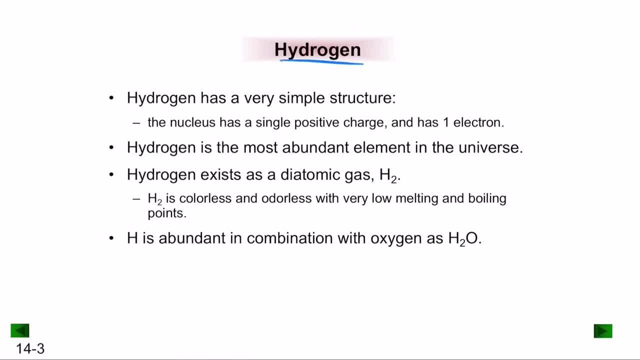 elements. So let's start with hydrogen. So hydrogen has a very simple structure. So this hydrogen molecule is a nucleus and has a single positive charge which has about one electron. Now, hydrogen is the most abundant element in the universe and it exists as a diatomic gas. 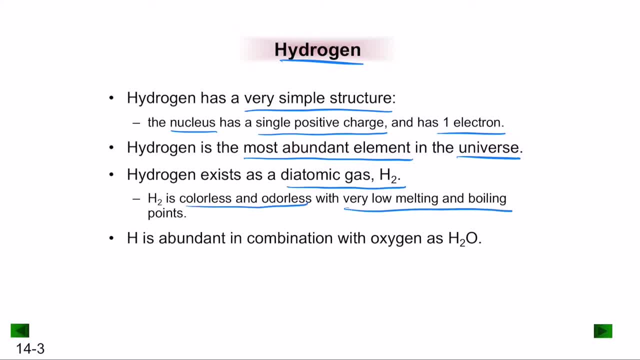 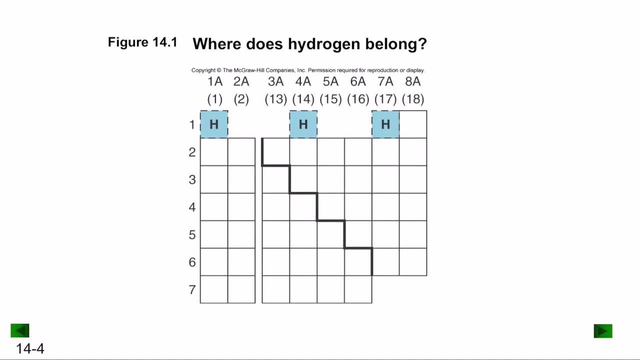 and hydrogen is generally colorless and odorless and has very low melting and boiling points, and hydrogen is abundant in combination with oxygen as H2O on the on the earth. So where does hydrogen belong? So hydrogen can be categorized into three category, three group elements based 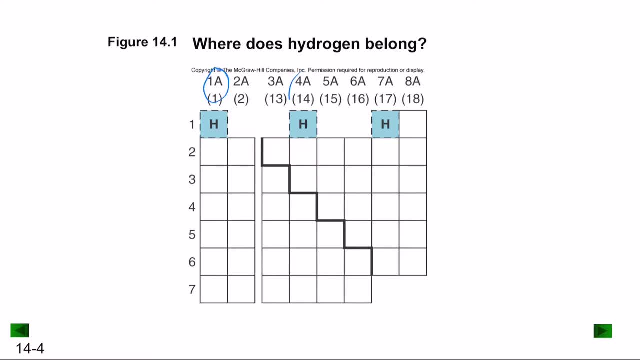 on its behavior. It can be a 1a group element, it can be a 4a group element or as well as it can be a 7a group element. So it can act as an alkali metal. it can act as a covalently bonded. 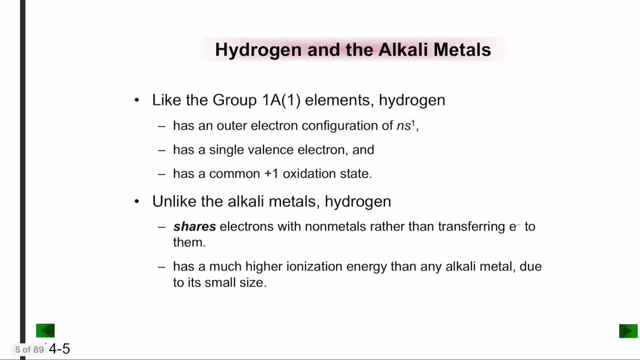 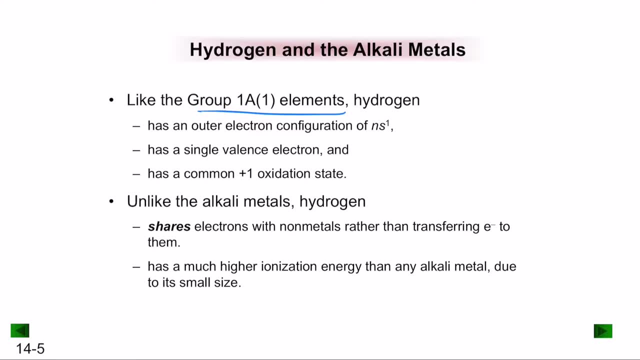 4a group element and it can also act as a halogen. So let's start with hydrogen and its similarity with alkali metals. So, like group 1a elements, hydrogen has an outer electronic configuration of ns1 and has a single valence, electron, and has a common plus one oxidation. 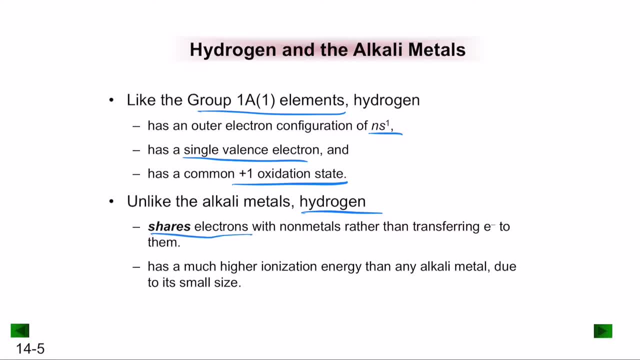 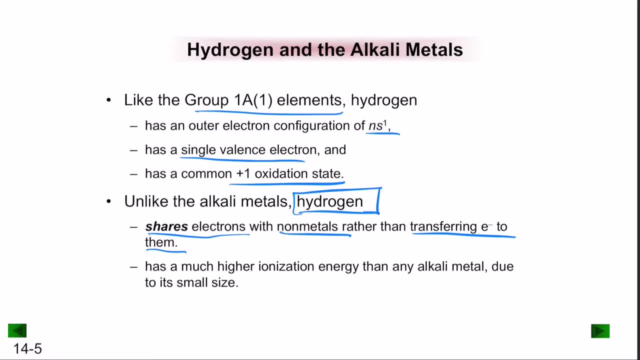 state. So, unlike the alkali metals, hydrogen shares electrons with non-metals rather than transferring electrons to them. So notice that hydrogen is the element that generally tries to share electrons, meaning that it generally covalently bonds with the electrons, with elements- rather than forming ionic bonds. Next, hydrogen also has a much higher ionization. 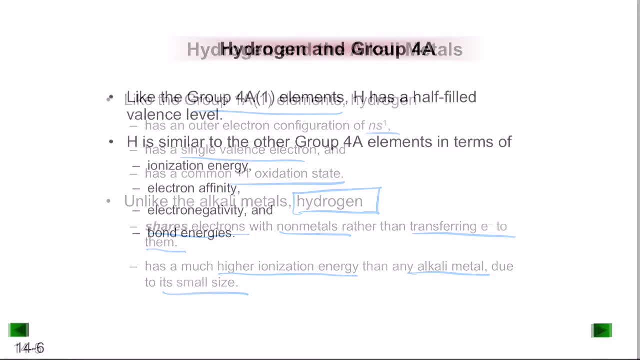 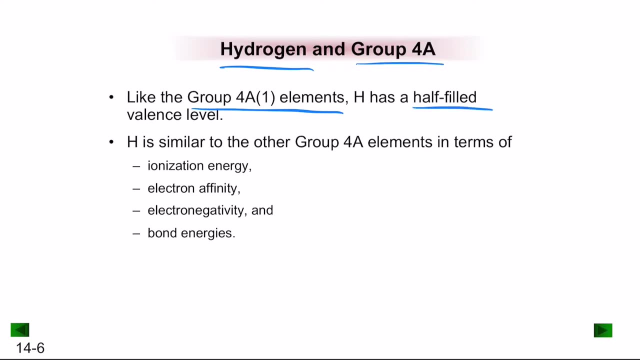 energy than any alkali metal due to its really small size. Next, let's discuss hydrogen and its similarity with group 4a elements. So, like the group 4a elements, hydrogen has a half filled valence level, So notice that it has two electrons. it's in the 1s valence shell, So notice that because it 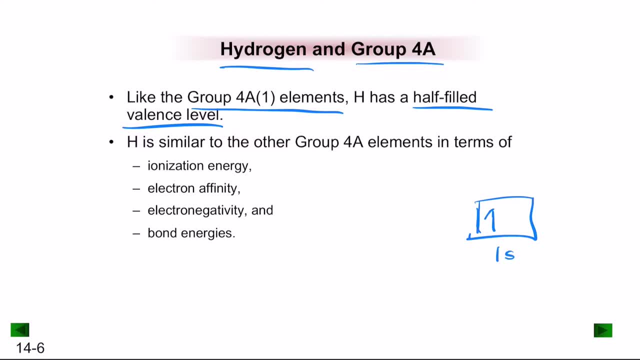 has only one electron filled, so which means that the entire orbit is half filled. So it's similar to 4a elements, but it is a half filled valence. So it's similar to group 4a elements, but it is a in terms of the ionization energy, electron affinity, electronegativity and bond energies. 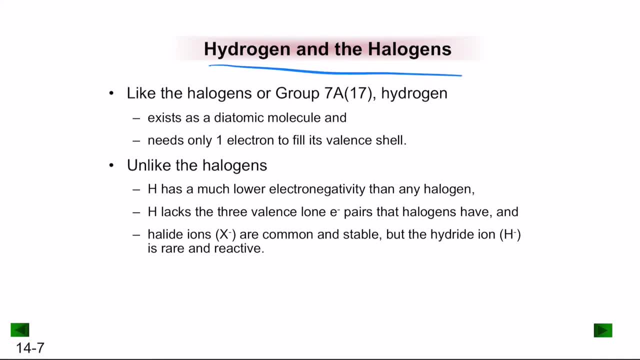 Next, hydrogen and halogens. So, like the halogens, hydrogen exists as a diatomic molecule and it needs only one electron to fill its valence shell And, unlike the halogens, hydrogen has a much lower electronegativity than any halogen. and 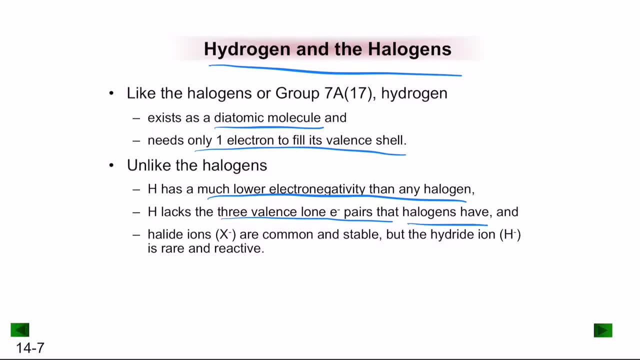 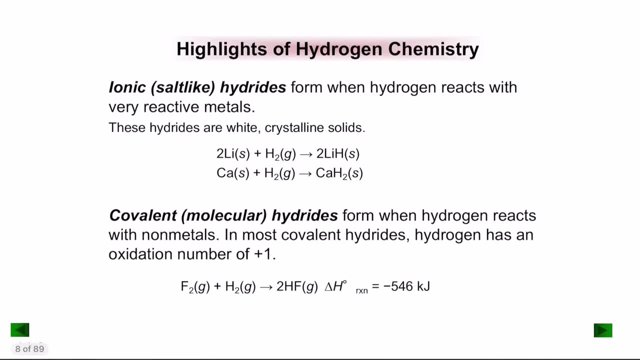 also lacks the three valence lone pair, lone electron pairs that the halogens have, And halide ions are generally common and stable, but hydride ions are rare and very reactive. So let's discuss some highlights of the hydrogen chemistry. Let's start with ionic hydrides. 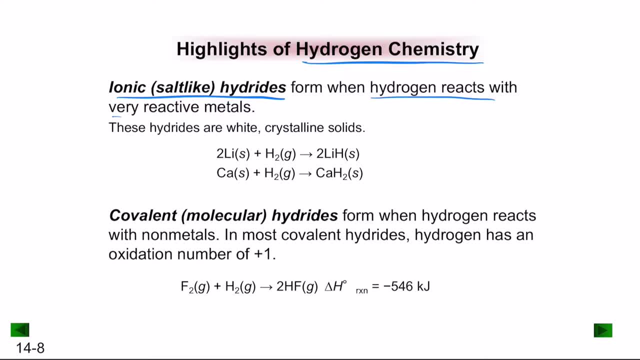 Ionic, meaning salt, like hydrides generally form when hydrogen reacts with very reactive metals, For example most commonly 1A group and 2A group element 2A group metals. So these hydrides are generally white and crystalline solids. 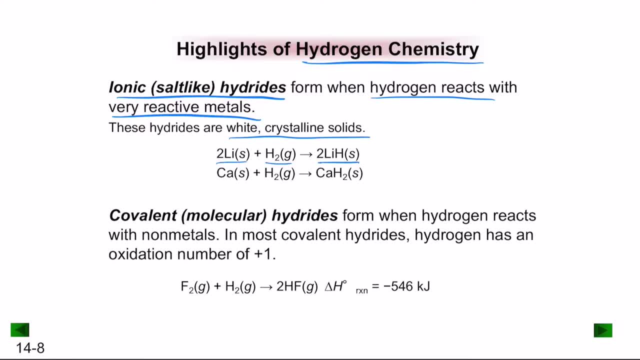 For example, when you mix lithium with hydrogen, it forms lithium hydride. When you mix calcium with hydrogen, it creates calcium hydride. Next let's discuss covalent molecule, covalent hydrides. So covalent hydrides form. 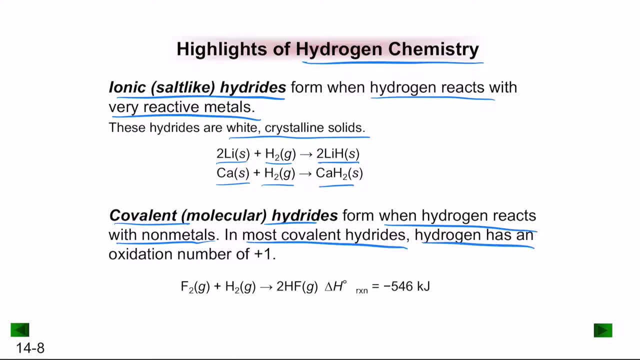 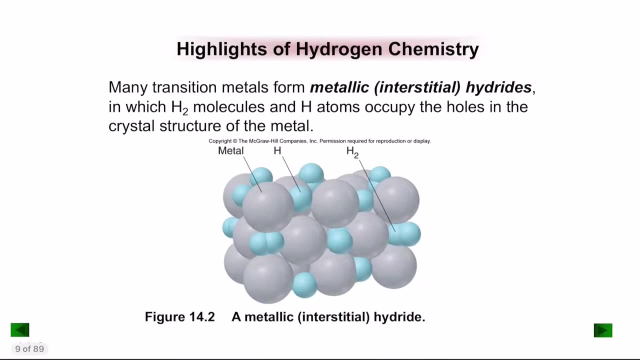 When hydrogen reacts with nonmetals, in most covalent hydrides hydrogen has an oxidation number of plus 1. So, for example, when you have fluorine reacting with hydrogen, it creates hydrogen fluoride, which has an enthalpy of reaction of negative 546 kilojoules, which is really high. 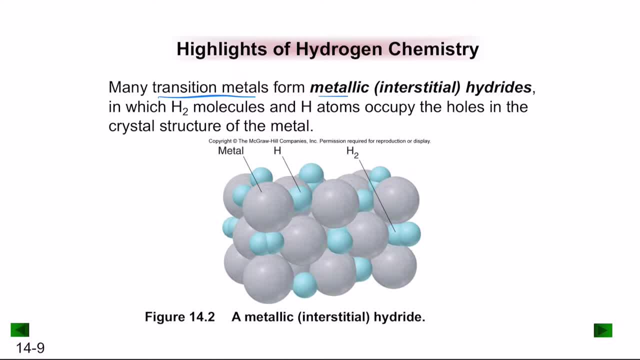 Now many transition metals also form what we call interstitial or metallic hydrides. This is where the hydrogen molecules will occupy the holes in the crystalline structure of the metal. So remember the term interstitial spaces. Interstitial spaces are the spaces between molecules. 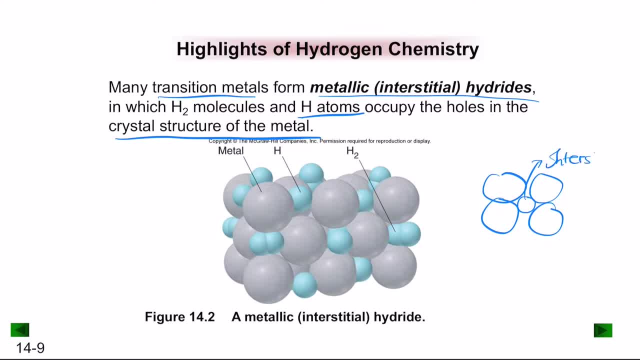 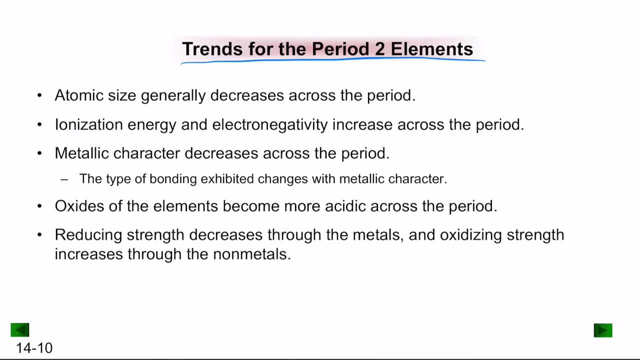 So this space here represents the interstitial space. So if the hydrogen molecule occupies the interstitial space, we call that an interstitial hydride or a metallic hydride. Next let's get into the trends for period 2. elements Now in period 2,. atomic size generally decreases across the period. 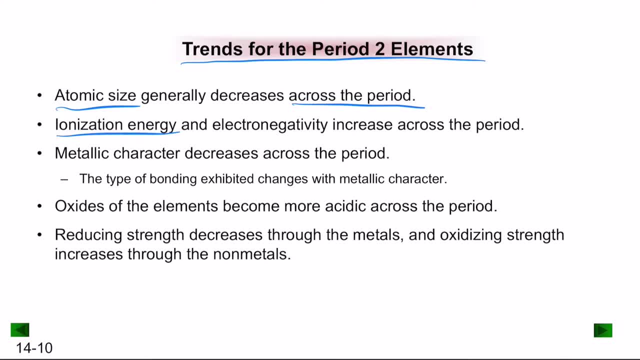 And ionization energy Because the atomic size decreases across the period, And ionization energy Because the atomic size decreases, ionization energy and electronegativity increase across the period And we notice that the metallic character generally decreases, meaning that you start. 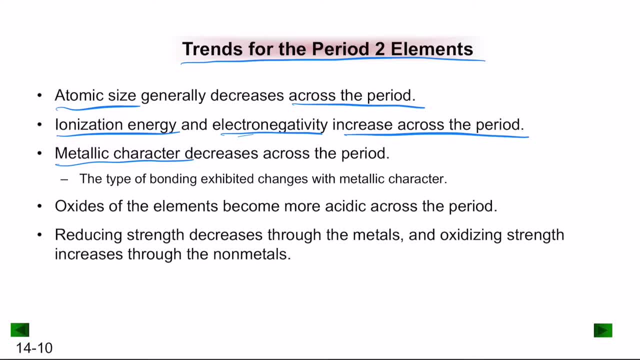 from going from a metal to a completely non-metal. So the type of bonding generally exhibited always changes with the metallic behavior. Next, oxides of the elements generally become more acidic across the period And finally, reducing strength decreases through the metals and oxidizing strength increases. 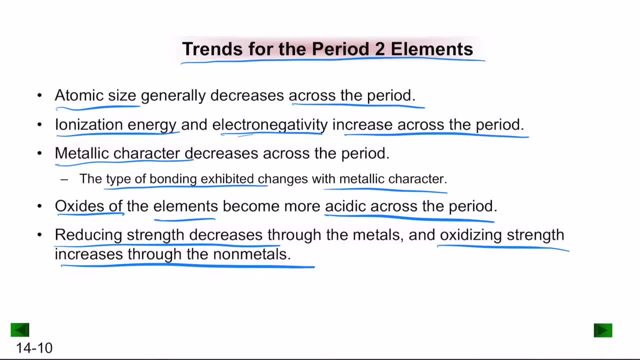 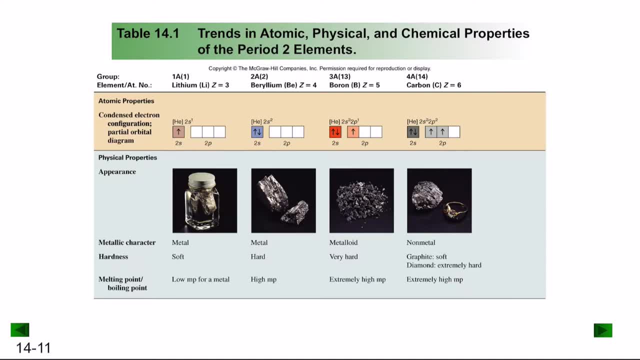 through the non-metals. So you go from a strong oxidizing agent To a strong reducing agent. So in terms of the material here you notice that as you go across the period you have a low melting point to extremely high melting points towards carbon. 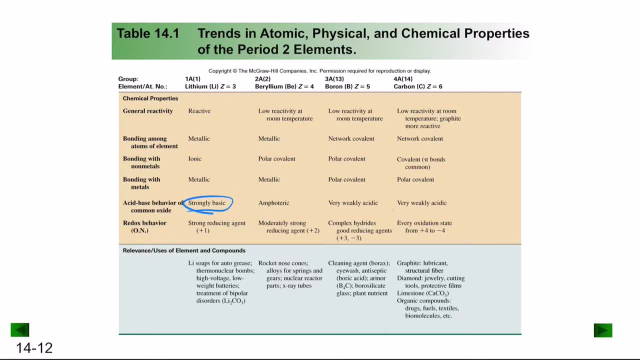 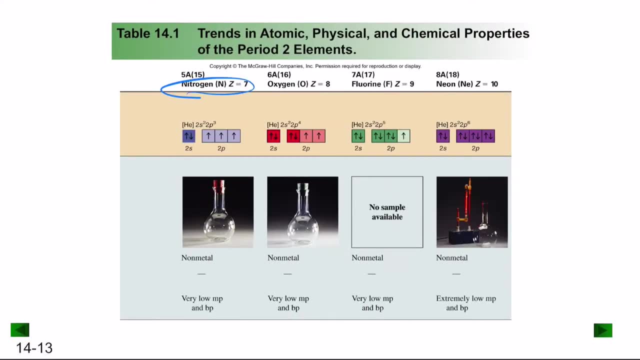 And you start from going from the behavior of being strongly basic to very weakly acidic towards carbon. But as you enter the realm of non-metals, where you start from nitrogen, so you start noticing that they have really low melting points and boiling points to extremely low melting points. 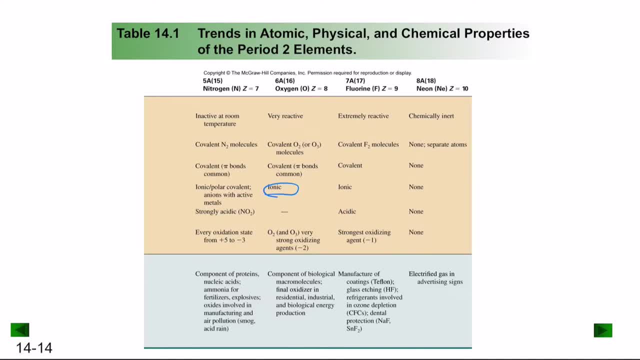 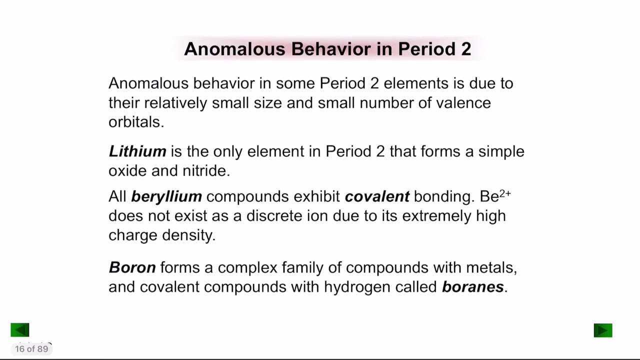 and boiling points And even the character generally becomes ionic to this active metal generally becomes none And they generally go from very reactive to chemically inert And you also have a strongly acidic character. So these are the trends in the period. two elements: 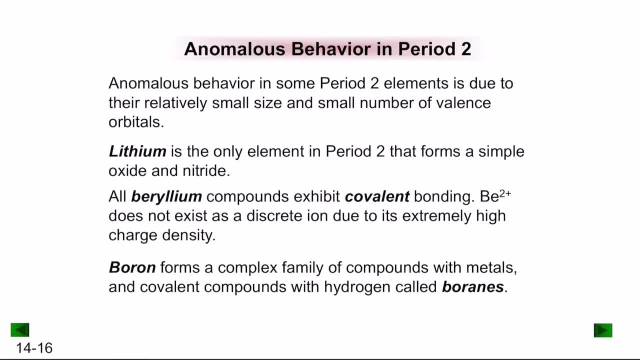 So what is the Anomalous behavior that we notice? So some of the anomalous behavior starts with lithium. So the reason it happens is because of the relatively small size and the small number of valence orbitals. So let's start with the lithium. 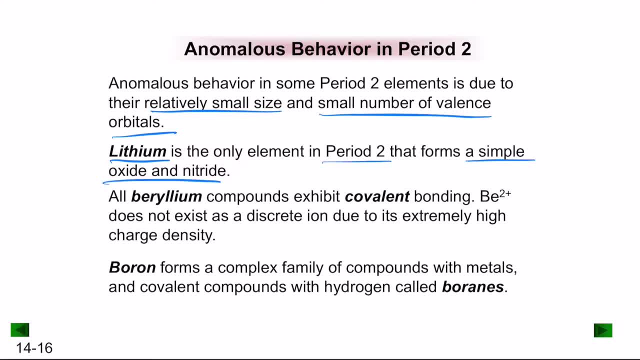 Lithium is the only element in period two that forms a simple oxide and nitrate. So all of the period two elements do not create, they form complex oxides and complex nitrites. Next you have all beryllium compounds. So beryllium is a compound that generally exhibits covalent bonding, even though it generally 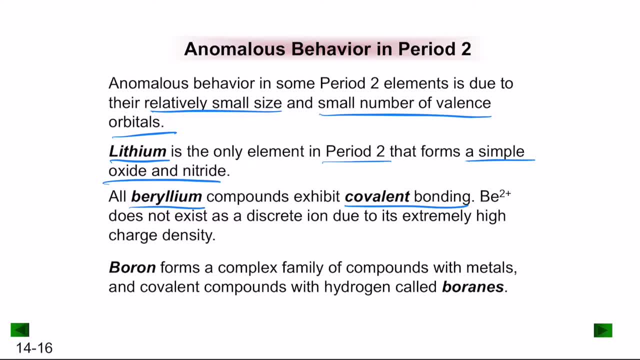 has, even though it generally is in the state of alkali and alkaline earth metals. So even though it's a metal, it doesn't exhibit bonding in terms of the metallic basis. The reason mainly is because that beryllium two plus does not exist as a discrete ion. 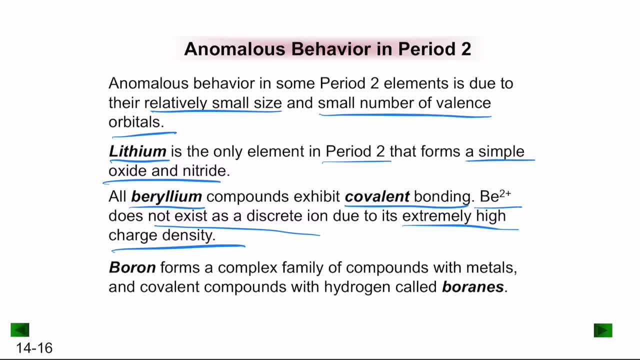 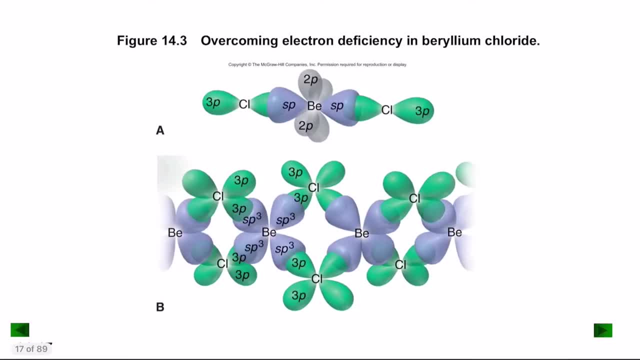 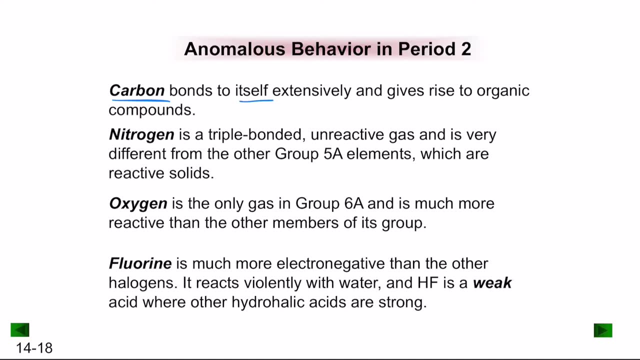 because it has a really high charge density. Next you have boron. that forms a complex family of compounds with metals and covalent compounds with hydrogens called borions. Now, Next one is carbon. So carbon is the only element that generally bonds itself extensively and gives rise to 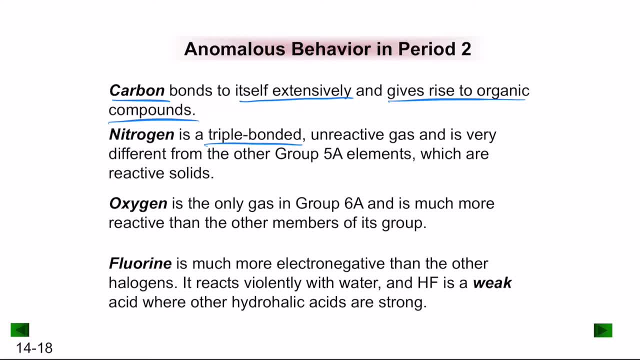 organic compounds. And you have a nitrogen that is triple bonded, unreactive gas and is very different from other 5A group elements, which are generally reactive solids. And you have the oxygen, which is the only gas in 6A and is much more reactive than other. 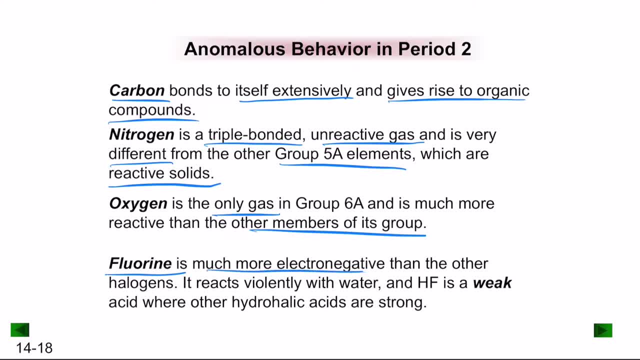 members of its group. Finally, we have fluorine, which is much more electronegative than other halogens, but it reacts violently with water And hydrogen fluoride is a weak acid, Whereas other hydrohylic acids are generally strong acids. So that is the anomalous behavior and the trends in period. two elements: 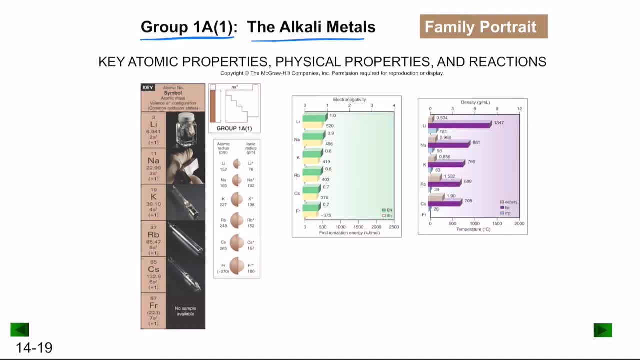 Next let's get into the group 1A elements. So group 1A elements, commonly called as the alkali metals, involve lithium, sodium, potassium, rubidium, cesium and francium. Out of these, we are mainly interested in the first five elements. 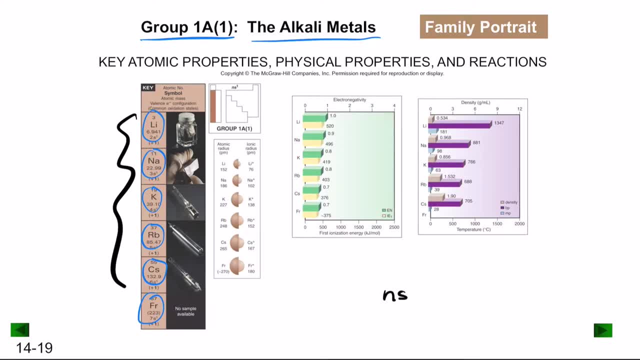 So all of these elements have a common configuration of ns1.. Common electronic configuration of ns1.. And they generally have an increase in the atomic size as you go across the group And there is a decrease in the electronegativity as you go across the group. 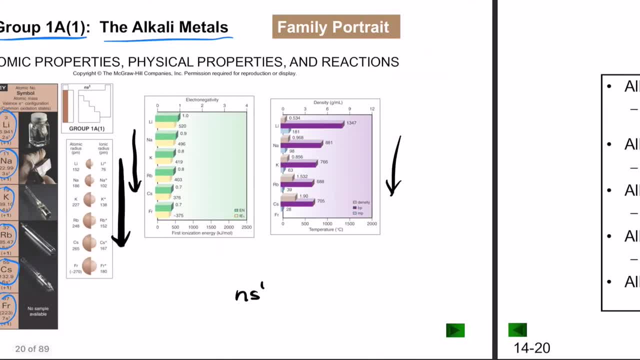 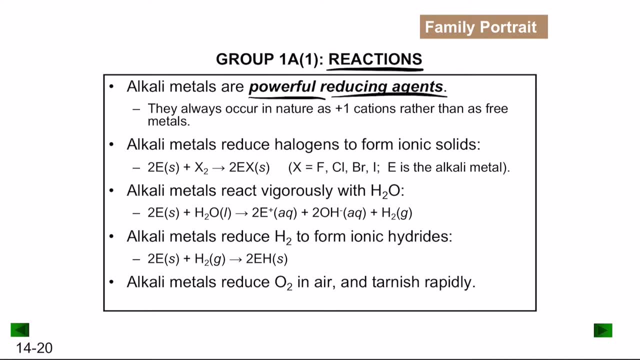 And also there is a decrease in the density of the metal. Now let's talk about some of the reactions of group 1A elements. So alkali metals are generally really powerful reducing agents And they always occur in the nature as plus 1 cations rather than free metals. 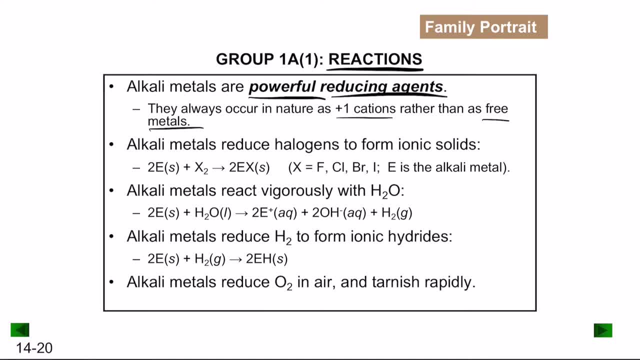 Remember that these are always existing as plus 1 cations. The reason mainly is because they always are ready to donate an electron. Now, alkali metals reduce halogens to form ionic solids. So when you have the alkali metal mixing with a halogen, 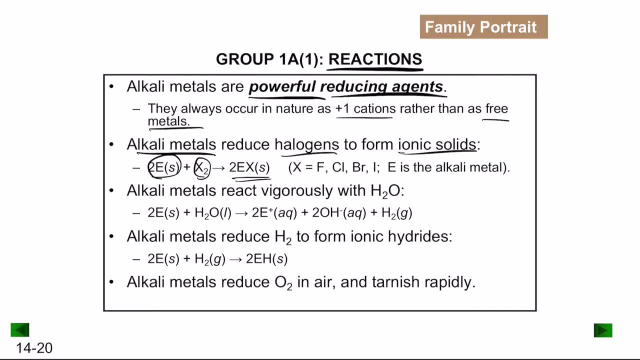 So that creates ionic solids, Ex. So Ex can be fluorine, chlorine, bromine or iodine, where E is the alkali metal, And alkali metals generally react vigorously With H2O, resulting in the production of hydrogen gas. So remember this: that when you put an alkali metal in H2O it releases hydrogen gas. 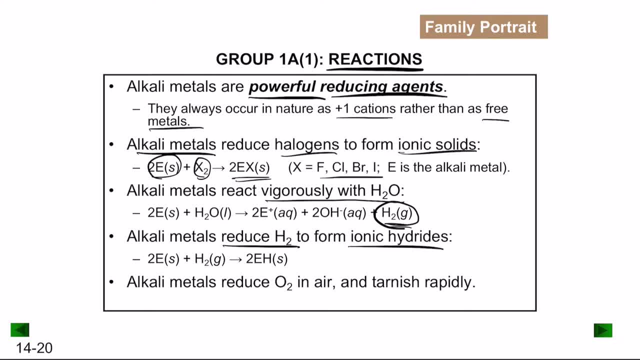 And also, alkali metals reduce hydrogen to form ionic hydrates. So when you mix an alkali metal with a hydrogen, it creates ionic hydrates. And finally, alkali metals reduce oxygen in the air and tarnish rapidly. That is the reason why alkali metals are generally stored in liquid medium, more commonly oil. 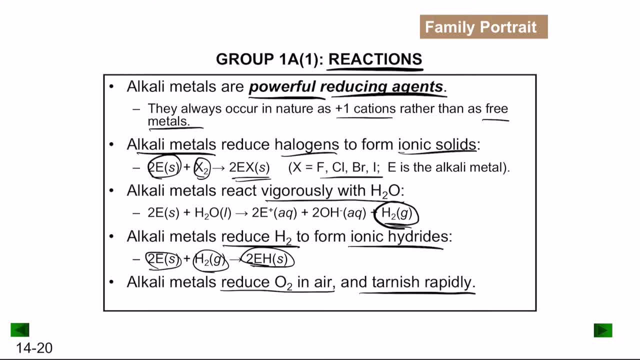 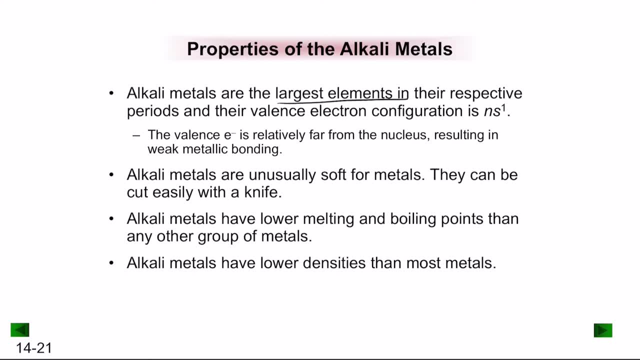 because it generally rigorously reacts with water, So it generally is stored in oil. Now let us look at some of the properties of alkali metals. So alkali metals are the largest elements in their respective periods And their valence electronic configuration is ns1.. 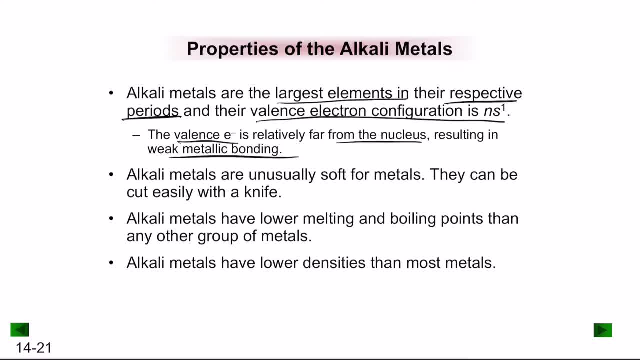 And this valence, electron, is relatively far from the nucleus, So resulting in a weak metallic bonding. So this is one of the reasons why metallic bonding is not common among alkali metals. That is the reason why they cannot exist as themselves, rather exist as cations. 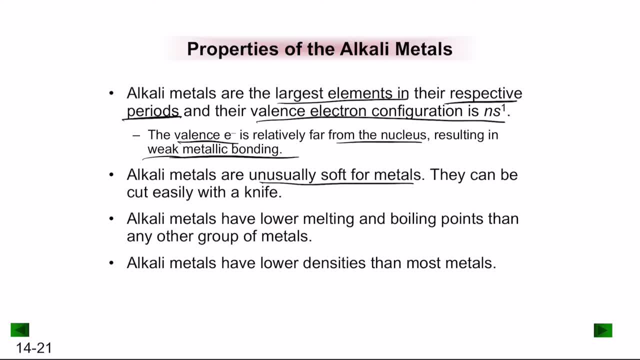 Now, alkali metals are usually unusually soft for metals because they can be easily cut with a knife. The main reason is because of the presence of weak metallic bonding, And alkali metals also have a lower melting and boiling points than any other group of metals. 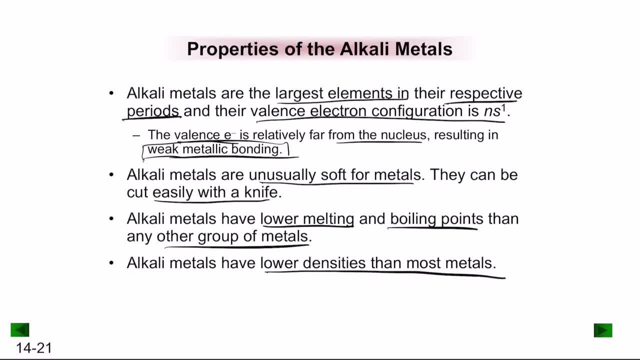 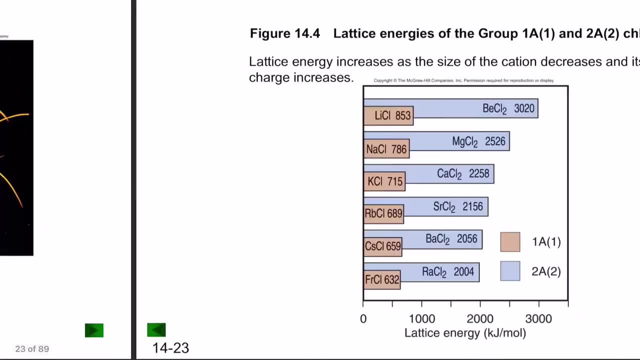 And finally, also have lesser doer densities than most metals. All of these can be contributed to the weak metallic bonding that exists in the structure. So let us look at some of the lattice energies of group 1a and 2a chlorides. 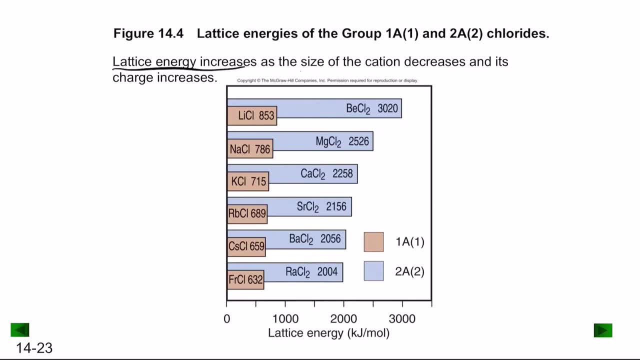 So we know the idea Here that lattice energy increases as the size of the cation decreases and its charge increases. So as the charge difference increases and the size of the cation decreases, there is a high increase in the lattice energy. That is why, even though lithium chloride has a really small amount of energy, beryllium 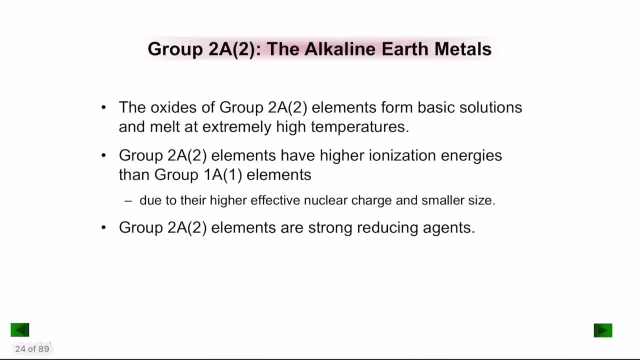 chloride has a really high amount of energy. So that is group 1a elements. Next let us get into group 2a elements, more commonly called as the alkaline earth metals, So the oxides. Oxides of group 2a elements generally form basic solutions and generally melt at extremely. 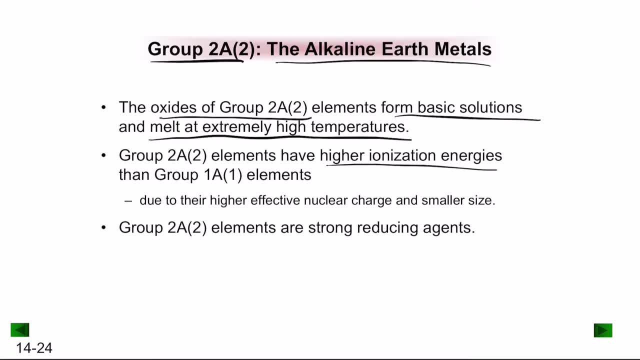 high temperatures And group 2a elements have generally have higher ionization energies than group 1a elements. The main reason is presence of 2 plus charge, So these are metals with E2 plus charge. The main reason is because of the higher effective nuclear charge and the smaller size. 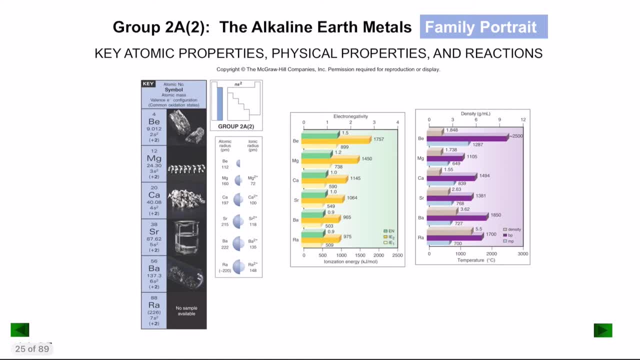 And finally, group 2a elements are also strong reducing agents, So these elements involve beryllium, magnesium, calcium, strontium, potassium and potassium. So these are the elements that are present in the group 2a elements. 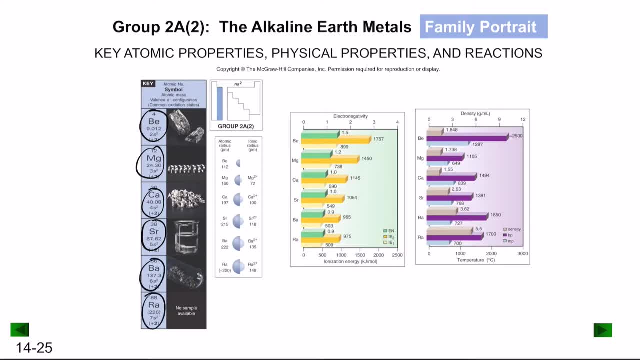 So these are the elements that are present in the group 2a: elements: Calcium, strontium, beryllium and radium. So again, atomic size increases, The same thing with electronegativity, decreases down the group and density varies differently. 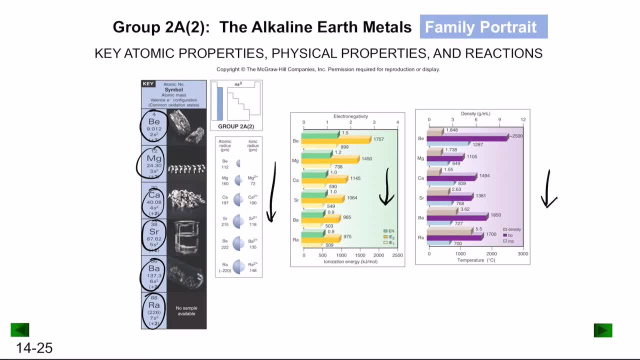 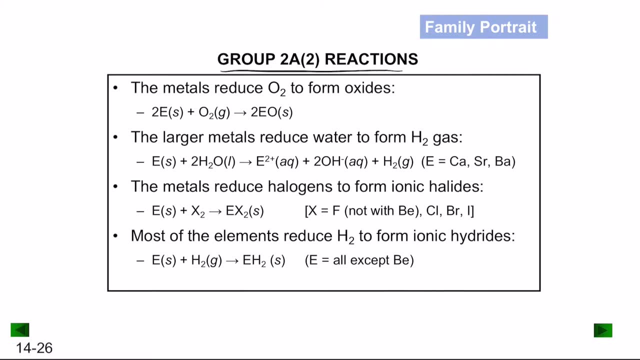 across the group. So density generally increases here as you go down the period. So the main reason is because of the increase in the atomic size. Next, let us talk about the reactions among group 2a elements. So again metals. These metals reduce oxygen to form oxides. 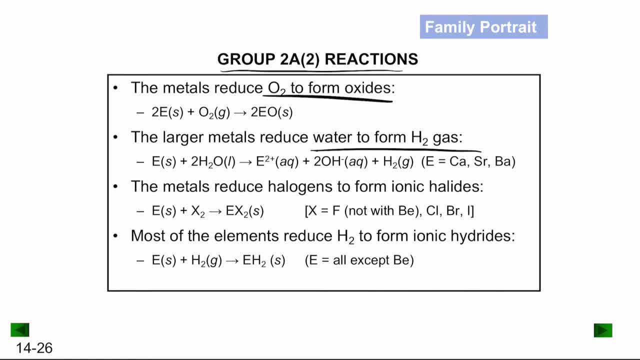 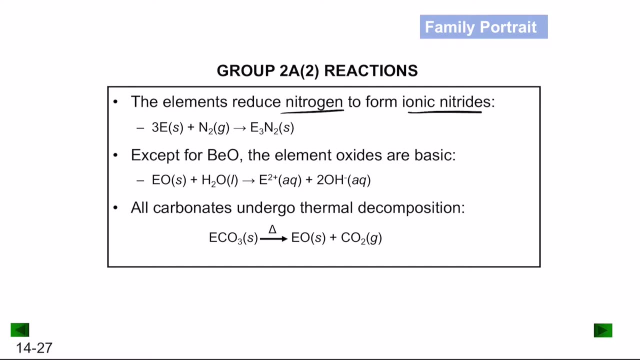 And they reduce water. They reduce water to form hydrogen gas And they reduce halogens to form ionic halides And they reduce hydrogen to form ionic hydrides. So these are the common reactions among group 2a elements. So, for example, when you react it with nitrogen, it generally creates ionic nitrides. 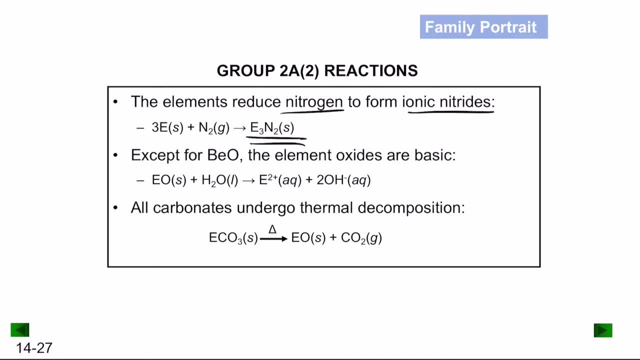 But a complex ionic nitrate called E3N2 nitrides. except for beryllium oxide, all of these elements are generally element oxides are generally basic, resulting in the production of OH- ions when you mix it with water And all carbonates undergo thermal decomposition. 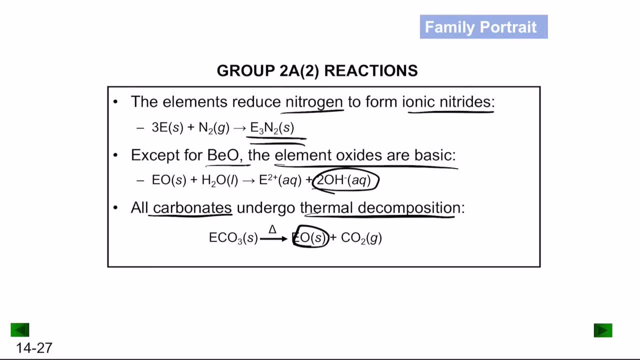 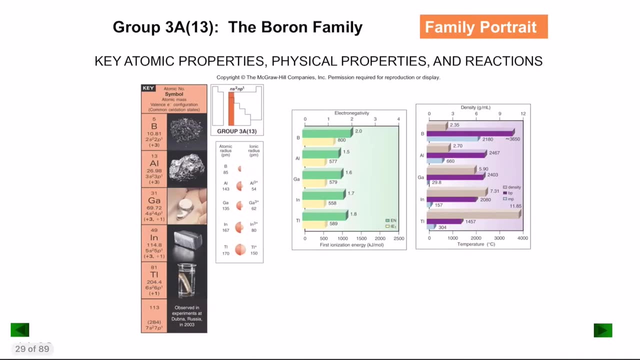 So thermal decomposition results in the formation of the metal oxide and carbon dioxide. So thermal decomposition results in the formation of the carbonates generally when under thermal decomposition release carbon dioxide for group 2a element carbonates. Next let us get into group 3a, elements. 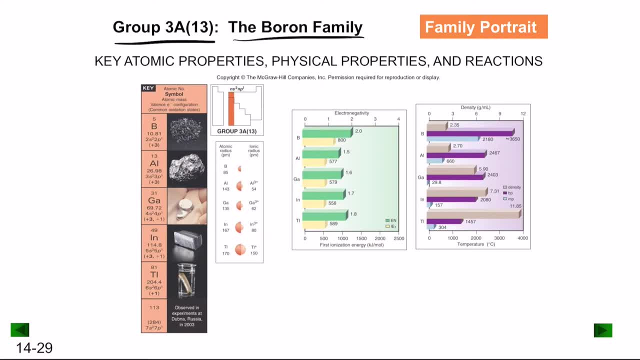 So 3a elements. The first one is the boron, So the commonly known as the boron family, So it starts with boron. aluminium, gallium, indium tellurium, and 113 is an element that generally is not observed and it hasn't been named yet. 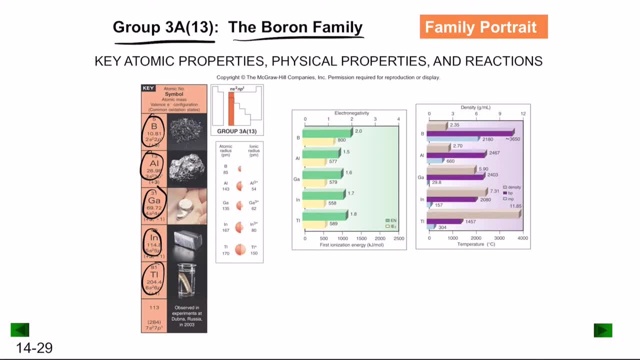 So let's get into the characteristics. So notice that all of these elements generally have general electronic configuration of Ns2Np1.. So these are the first elements in the p-group elements, And their ionic atomic size increases as you go down the group. 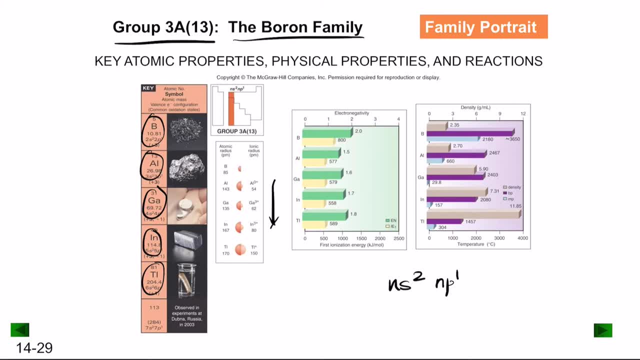 And their electronegativity generally varies differently as you go down the group. The main reason is because you go from a metalloid to a metal. So you are going from a metalloid to a metal, So this results in a higher electronegativity as you go down the group. 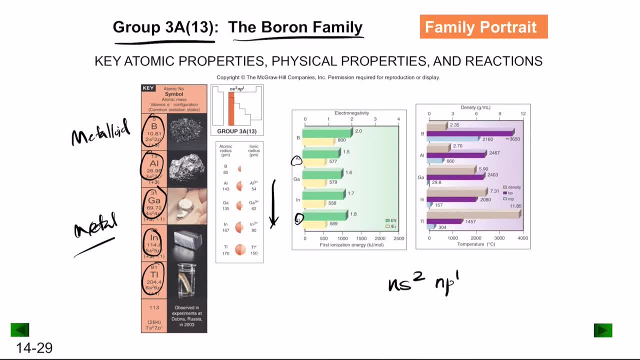 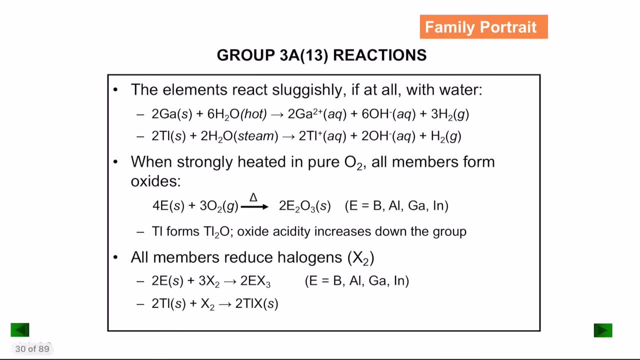 From aluminium to tellurium, there is an increase in their electronegativity. Next let us go to the reactions. So So these elements react sluggishly, if at all, with water, So which means that these need the water to be either in the form of hot water or steam. 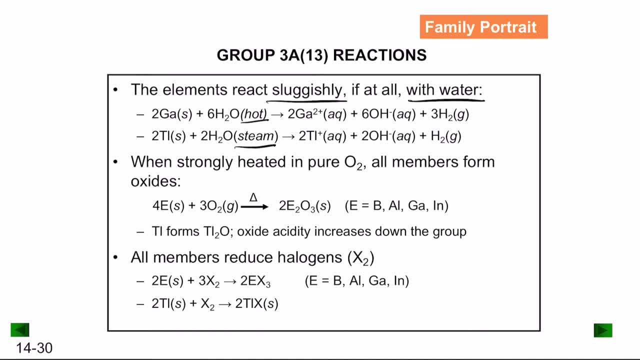 Only then. these elements generally react with water, resulting in the production of hydrogen gas, But the reacting normally is not something that happens So, which means that they are slow to react with water And they, when you heat it strongly, in pure oxygen all members generally form oxides. 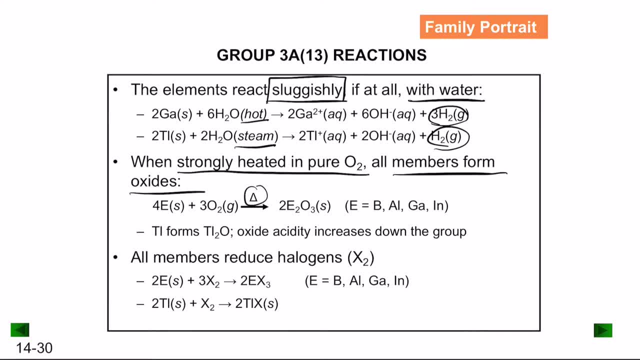 But it requires a certain amount of heat. Ok So, but tellurium also forms tellurium oxide and oxidized acidity increases down the group. Next, all members reduce to halogens. So when you mix it with halogens it creates halogen. 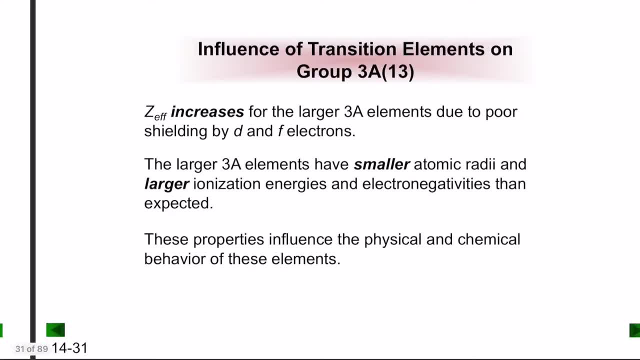 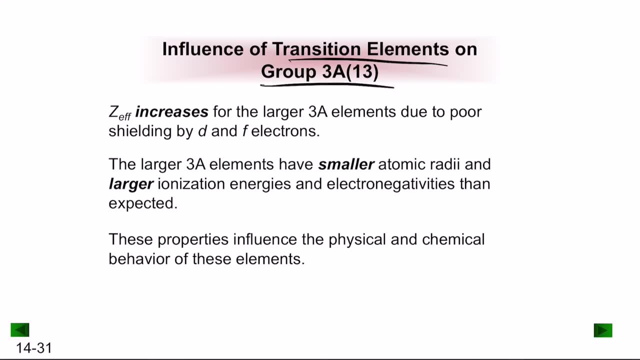 So they undergo reduction with halogens and generally create halogens. Next, let us talk about the influence of transition elements on group 3a elements. So in group 3a, why do they have something different? here is the presence of group 3a. 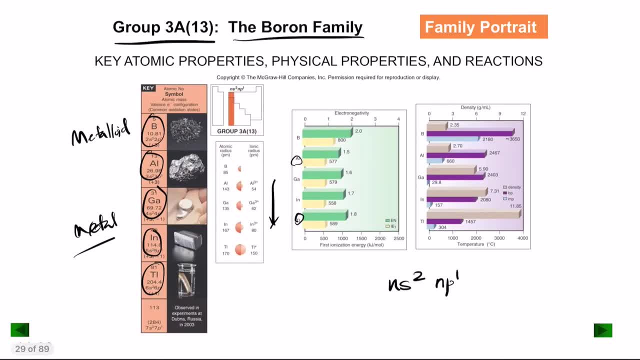 the transition elements As you go beyond aluminium, So from aluminium when you enter into gallium, indium and tellurium. all of these three elements are generally elements that come after the transition elements, So which means that they do have a D sub shell. 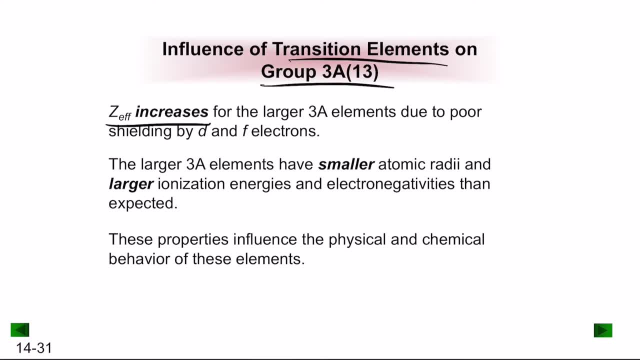 So because of the presence of that D sub shell, it increases the effective nuclear charge for the larger 3a elements due to poor shielding by D and F electrons. And finally, the larger 3a elements generally have smaller atomic radii and larger ionization. 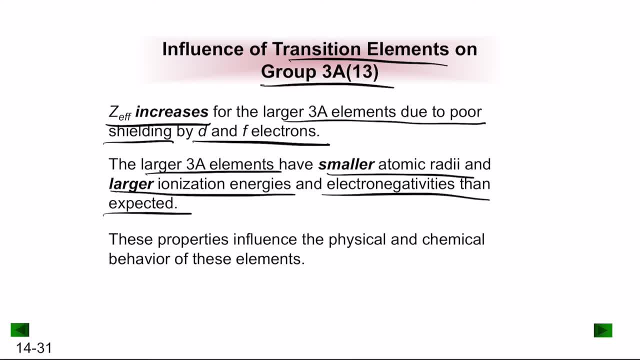 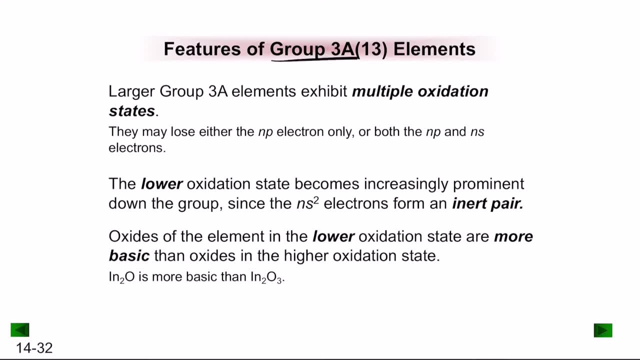 energies and electronic activities than expected, And these properties can influence the physical and chemical behavior of these elements. So what are the features of group 3a elements? So larger group 3a elements exhibit multiple oxidation states. So this is one of the important parts to remember. 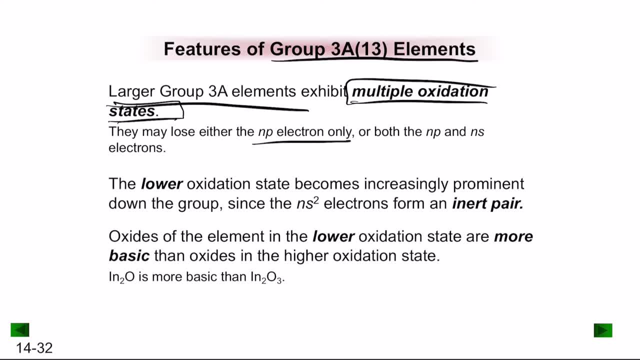 The main reason is because they can not only lose the electron in the NPE, but they can lose both the NP and NS electrons at the same time, resulting in either plus 3 or plus 1 oxidation states. So this can be in any form, of any form possible. 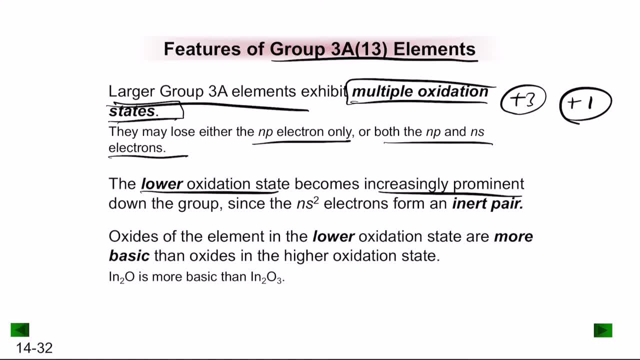 So let us look at the next slide. The lower oxidation state becomes increasingly prominent down the group, since the NS2 electrons form an inert pair. and finally, the oxides of elements in the lower oxidation states are generally more basic than oxides in the higher oxidation states, which means that indium 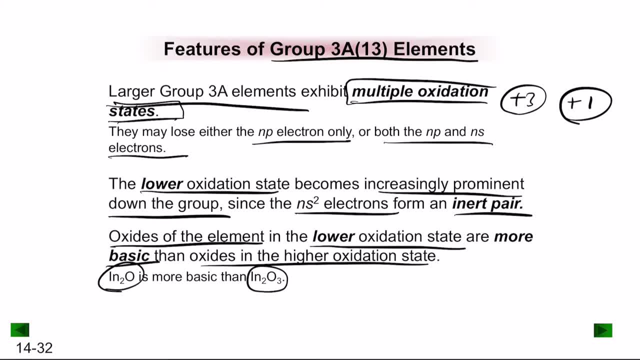 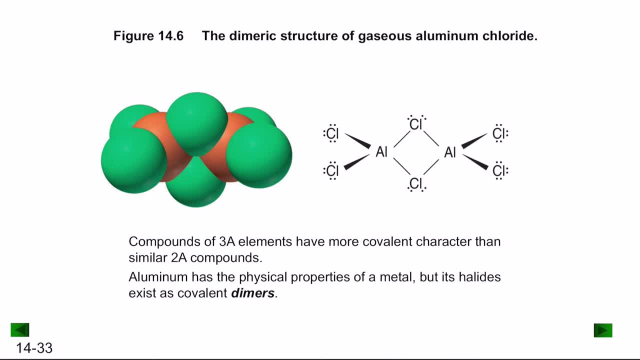 oxide is more basic than indium trioxide. Aluminium also creates dimeric structures, So which means that this creates what we call dimers, So where the compounds of these 3a elements, These 3a elements have more covalent character than similar 2a compounds. 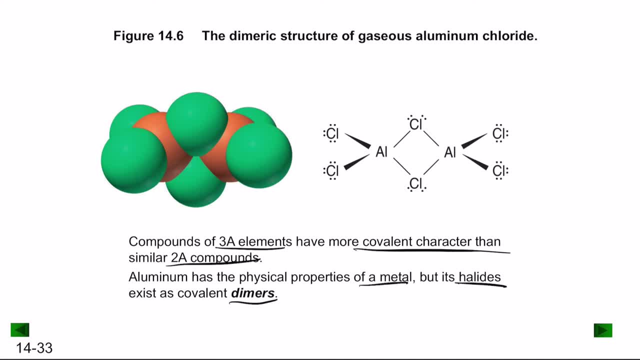 So aluminum has the physical properties of metal, but its halides can exist as a covalent dimer. So covalent dimer here means that aluminum can create four bonds and create a metal structure that looks something like this: So rather than existing as an electron deficient aluminum trichloride- 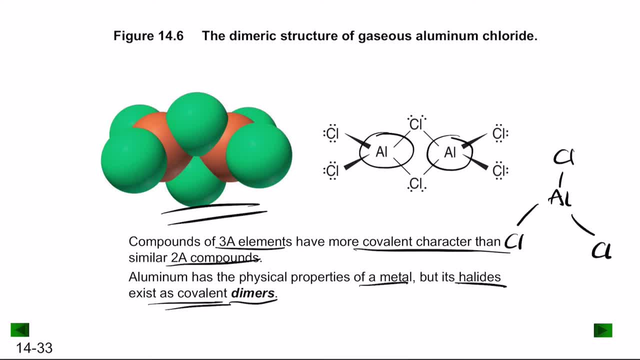 So rather than existing as an aluminum trichloride, So it creates dimers where it bonds, So the same chlorine Is being shared by two aluminum atoms, creating what we call as a dimer. So the term dimer comes because of the presence of two separate aluminum trichloride molecules. 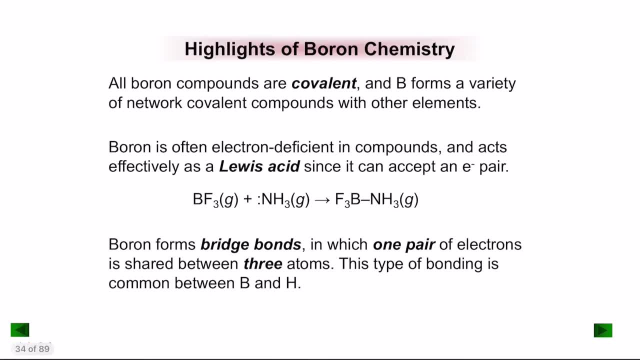 combining to create a single structure. Next, let's talk about boron. So all of these boron compounds are generally covalent and boron forms a variety of network covalent compounds with other elements. Why does this do that? The reason is because it is electron deficient. 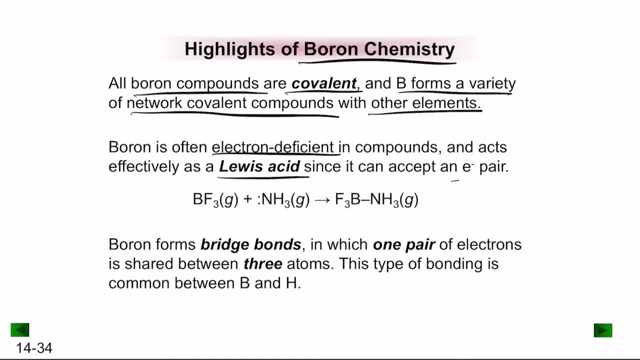 Because it's electron deficient. It acts as a covalent, So it's a covalent compound. It acts as a Lewis acid because it always tries to accept an electron tape, So resulting in the formation of what we call bridge bonds. 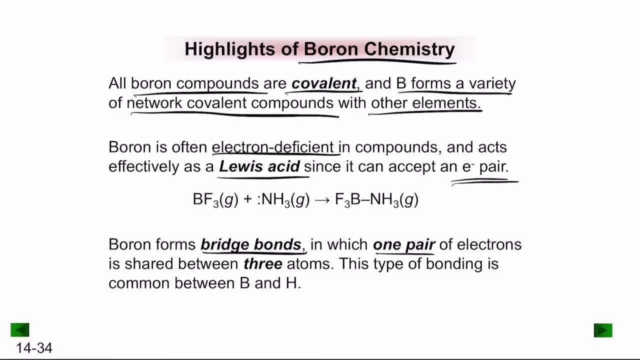 So bridge bonds is where only one of these. So when we consider what is a bridge bond here, Let's consider boron, trichloride and ammonium. To create a bond between these two, for generally a covalent bond, both have to share the electrons. 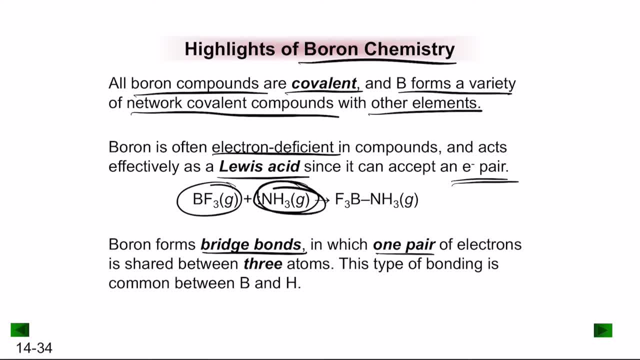 Rather than both sharing the electrons, if only one element shares the electrons while the other does not share any electrons. That type of a bond is generally called as a bridge bond Right, And it's generally being shared by three atoms, and this type of bonding is generally common. 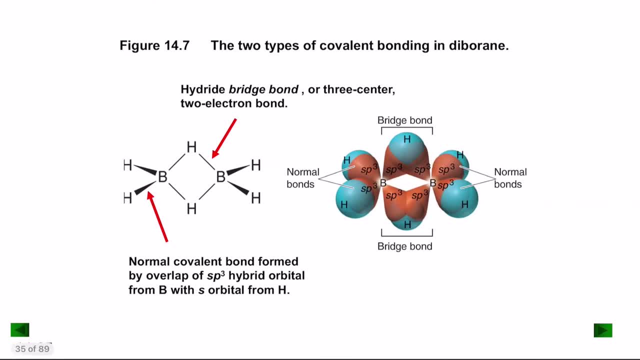 between boron and hydrogen, resulting in the formation of diborane. So diborane is a structure that looks somewhat like this. Remember, generally borane is BH3.. So, which means that boron generally only has three bonds, while being electron deficient because it only has six electrons in its surrounding shell. 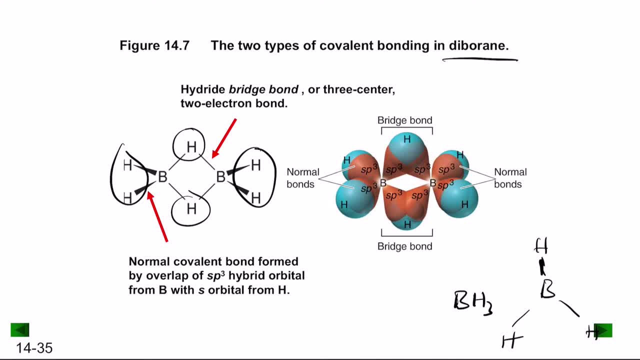 So it creates similar to dimers among aluminum trichlorides. The same thing happens with BH3. Boron trihydride, resulting in the formation of diborane. So these bonds here are generally called as the bridge bonds. So these are bonds which are donated by one atom rather not being donated by both atoms. 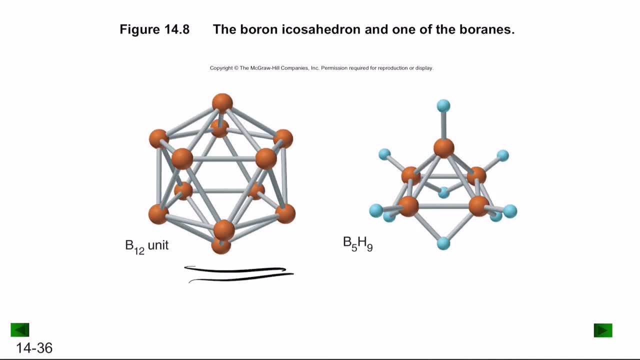 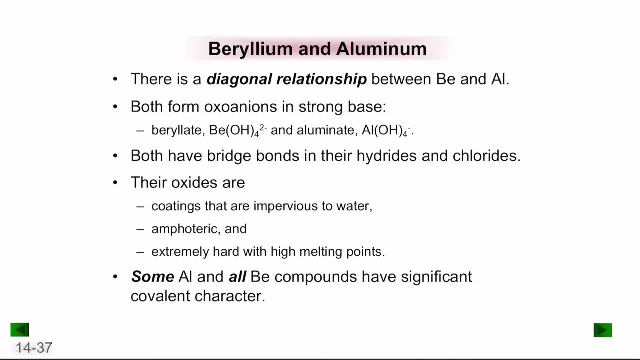 So this can create peculiar structures where you have boron, icosahedron and one of the boranes which can be B5H9 or B12 unit system. Next, let's discuss beryllium and aluminum. So there is a diagonal line. 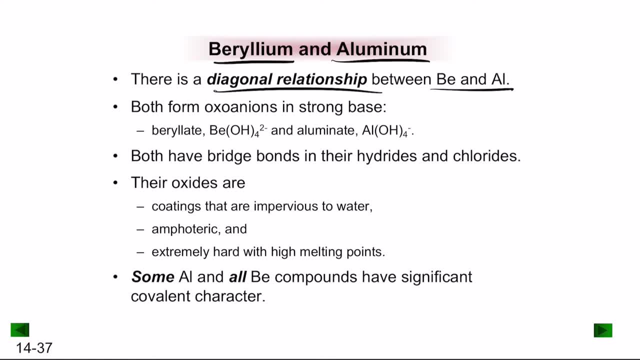 So there is a diagonal relationship between beryllium and aluminum, So meaning that both of these form oxo ions in a strong basis, where they create beryllium hydrate and aluminum hydrate, aluminate- So generally beryllate and aluminate- and both of these have bridge bonds in their hydrates. 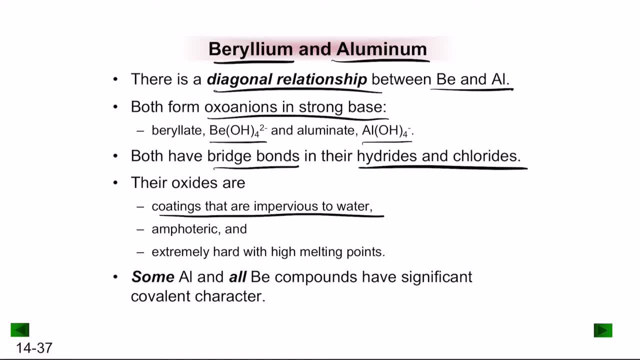 and chlorides and their oxides are generally coated. their oxide coatings are generally impervious to water. they are amphoteric and extremely hard with high melting points, And some aluminum and all beryllium compounds have significant covalent character. 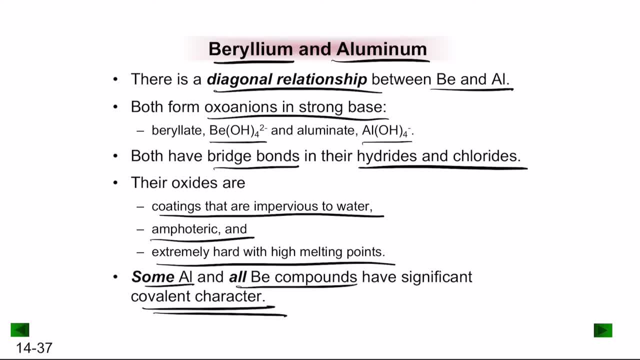 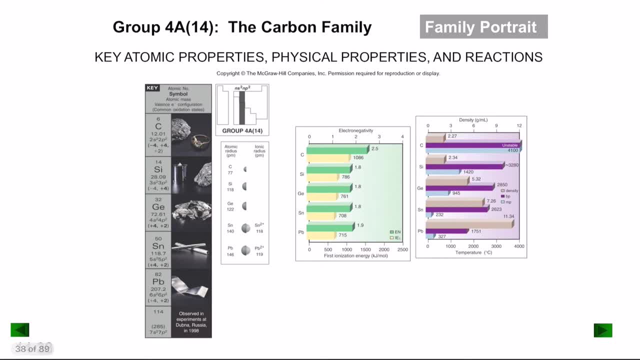 Even though aluminum is a metal, it can act with high amount of covalent character, resulting in the formation of dimers, as we saw before. So with that we end the discussion on group 3 elements. Next, let's get into group 4A, more commonly known as the carbon family. 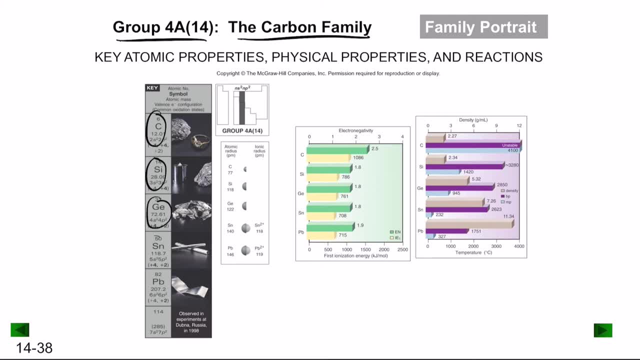 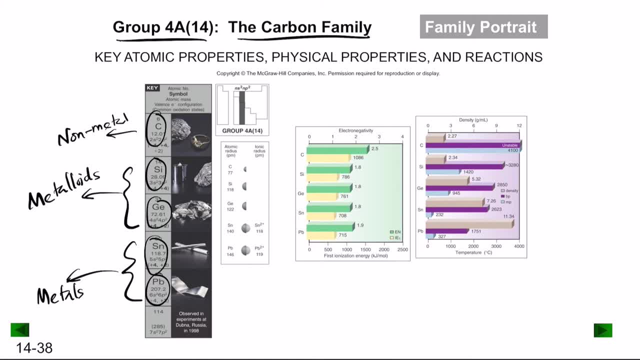 Notice that this behavior is something peculiar across different spaces. You notice that you are going from a non-metal to a metalloid, to a metal, So that's why this is a special group. The main reason is mainly because of the presence of ions when you go into lead, tin and lead. 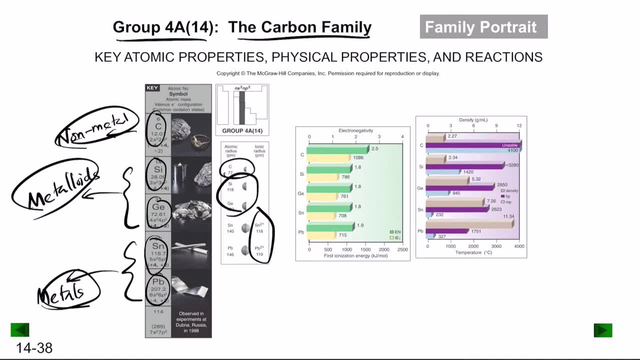 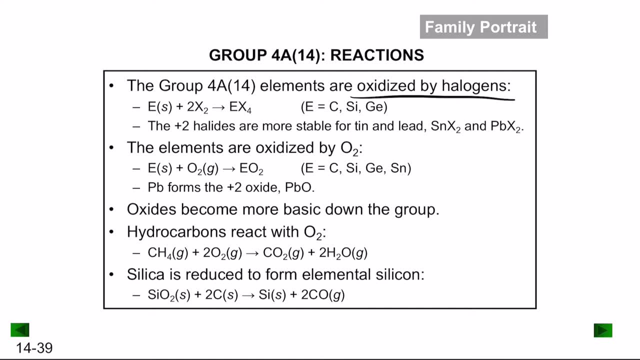 While silicon and germanium have a significant covalent character and carbon only creates covalent bonds. Now let's get into the reactions. So group 4A elements are generally oxidized by halogens, More commonly carbon, silicon and germanium. 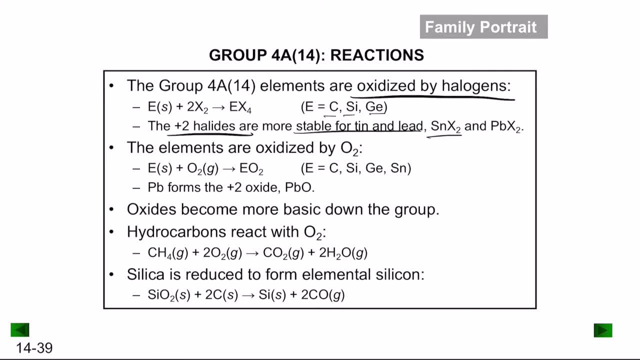 And all the plus 2 halides are more stable for tin and lead, resulting in the formation of SnX2 and PbX2.. Next, we have elements that are oxidized by oxygen. So when you mix it with oxygen, they create oxides. 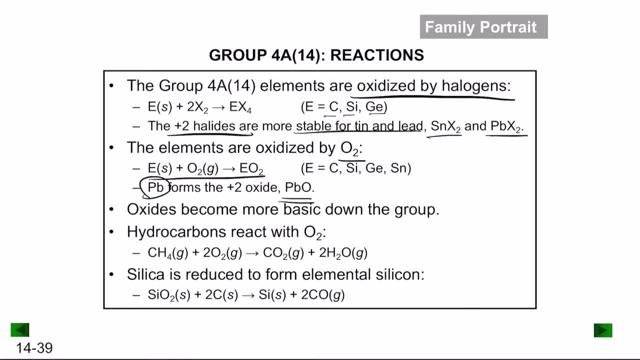 But when lead does that, it creates lead, So that's why it's called covalent bonds. Lead oxide, PbO Oxides are generally more basic down the group And hydrocarbons can react with oxygen, resulting in the production of carbon dioxide. 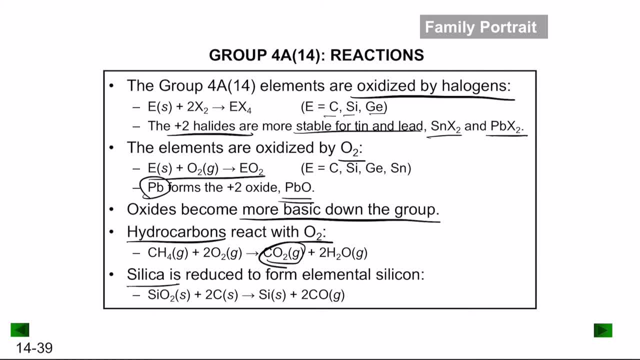 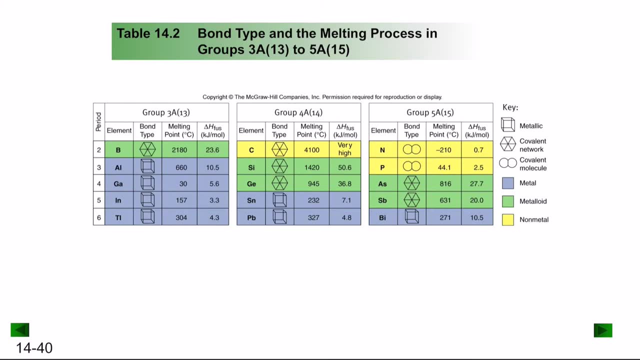 And silica, which is SiO2, is reduced to elemental silicon when you mix it with these compounds. So when you mix it with carbon, results in the formation of silica and carbon oxide. So let's look at the bond type and the behavior of these elements. 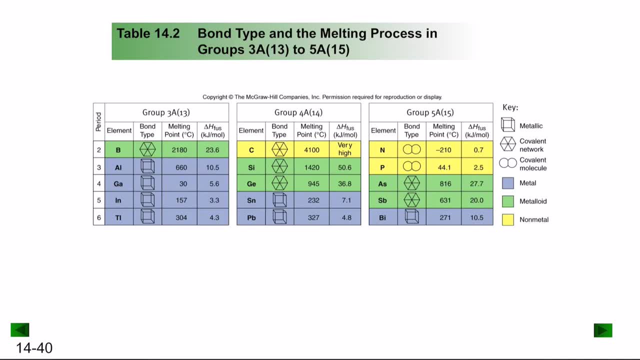 Especially in terms of their fusion energy. So when you look at group 3A elements, you start with a non-metalloid which has a really high melting point towards a carbon material which generally also has a high melting point to. you go into nitrogen group 5A element, which generally can be a gas, towards arsenic and 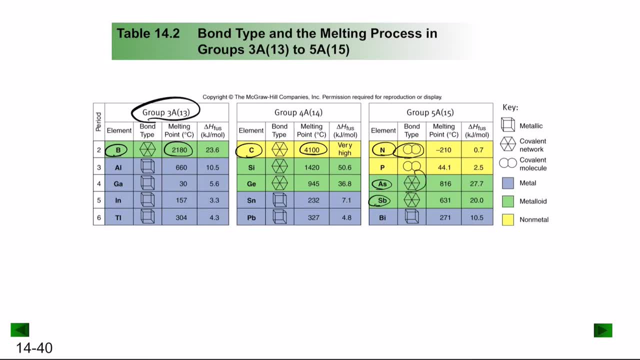 lead, So arsenic, and stromal, which generally, again, is a metalloid. So notice that as you go across these elements, You start with a non-metalloid which has a really high melting point, Towards a carbon material which generally also has a high melting point. 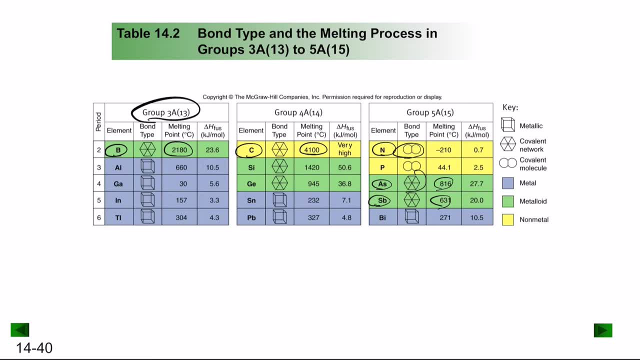 And across 3A, 4A and 5A, you start going towards non-metals, where carbon, nitrogen and phosphorus are non-metals, while silicon, germanium, arsenic and boron- all of these are elements that are metalloids. 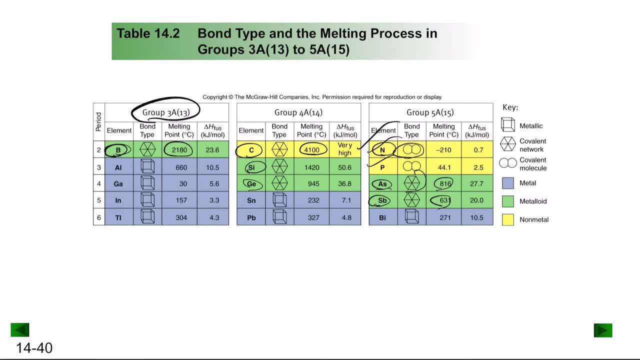 And you go into metals, which are always there. When you enter into 6A and 7A, you start noticing that there is no metals at all. So the type of bond that creates metalloids generally have a covalent network bonds. 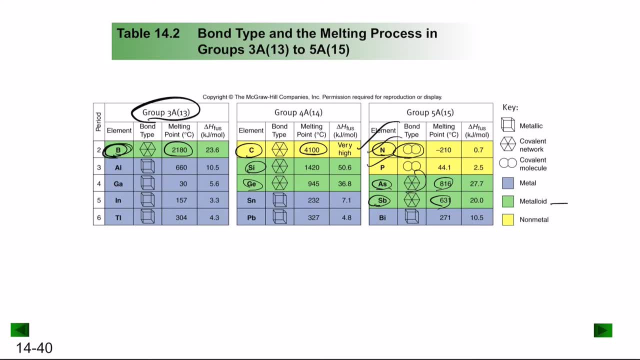 So metalloids Generally have covalent network bonds, while non-metals have covalent bonds, Metals have metallic bonds. There are some non-metals that can also be considered for a covalent network bond, So one among them is carbon. 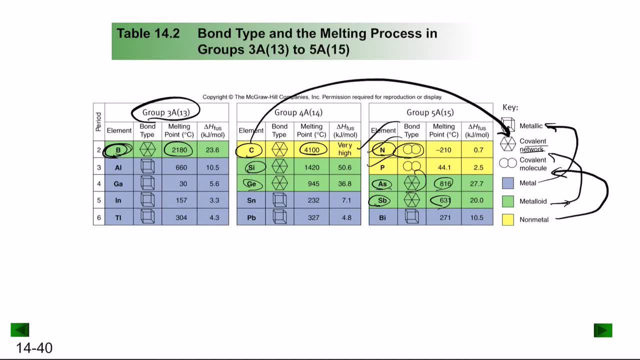 So the more commonly known element that can create a network covalent bond among carbon is diamond, creating a network covalent structure even though it is a non-metal. So this is a covalent bond. This is a covalent bond. 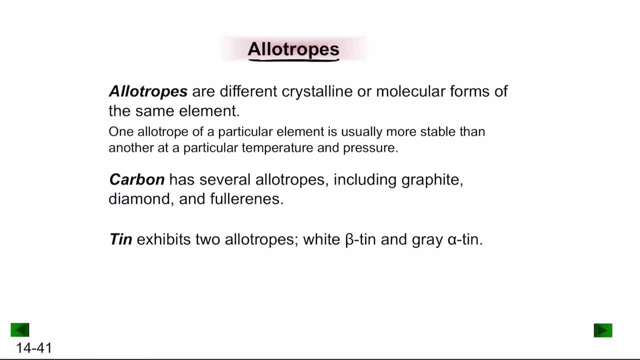 This is a covalent bond. Next, let us talk about another property of 4A group, elements called allotropes. So allotropes are different crystalline or molecular forms of the same element. So one allotrope of a particular element is generally usually more stable than another. 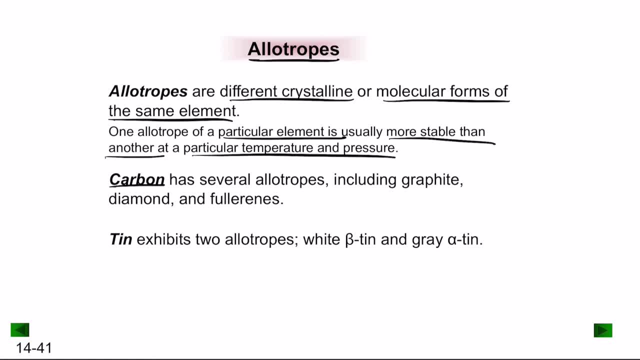 at a particular temperature and pressure, For example. carbon has several allotropes. For example, one of them is graphite. Second is diamond. The third is fullerenes. Graphite has a smoother structure. Diamond is a more rigid structure. Fullerenes is also a more rigid structure. 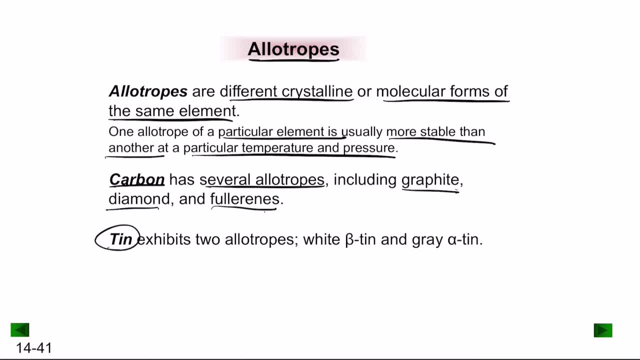 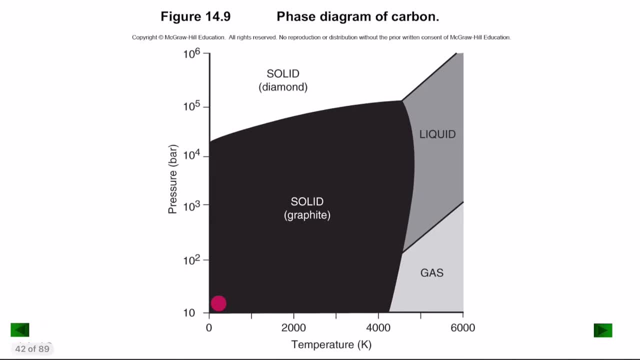 You can also take the same example for tin. Tin also exhibits two allotropes: One is a white beta tin and a gray alpha tin. So this is one peculiar property of 4A group elements. So let us look at a weight diagram for carbon. 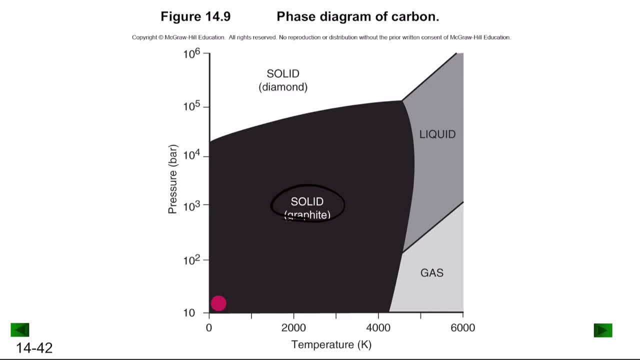 At lower pressures and lower temperatures they exist. So carbon exists as graphite, But at extremely high pressures it exists as a solid. So when you have so it ranges around 5000 Kelvin, At around 1000 Kelvin, At around 1000 Kelvin. 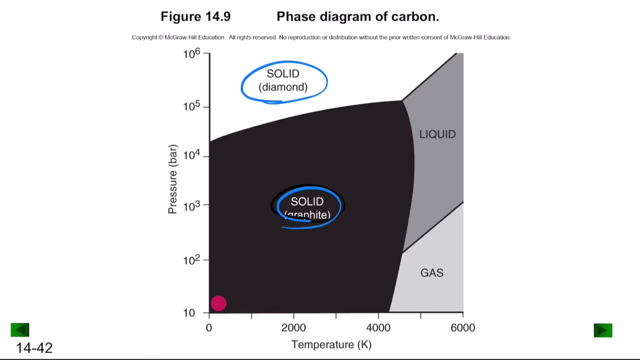 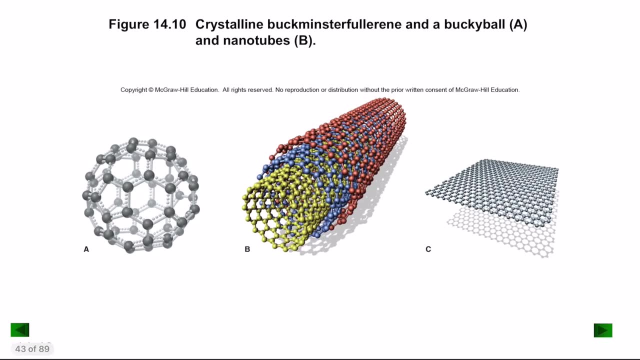 At a pressure of about 10 to the power 4 bar. it exists as diamond, But anything above that. it enters into liquid and gaseous phases. So these are different structures that can be created with Buckminster fullerene, which is an allotrope of carbon. 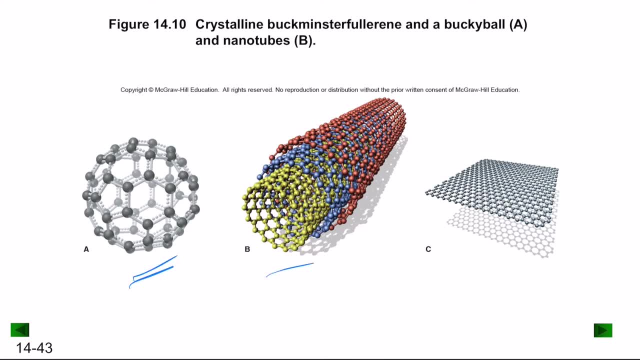 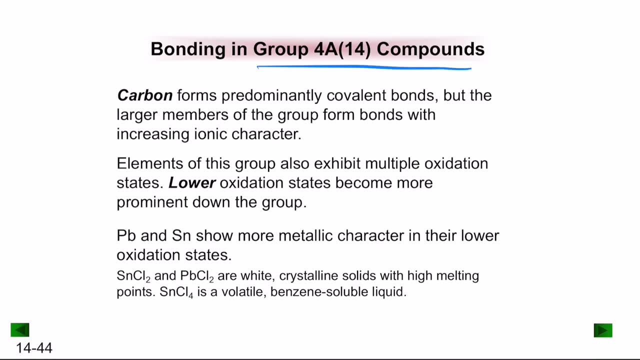 So, which can create a circular structure, nanotube structures and a sheet structure. So let us look at bonding in group 4A, elements, So carbon, generally predominantly covalent bonds. It does not have any other type of bonds, But as you go to the larger members of the group they form more ionic character bonds. 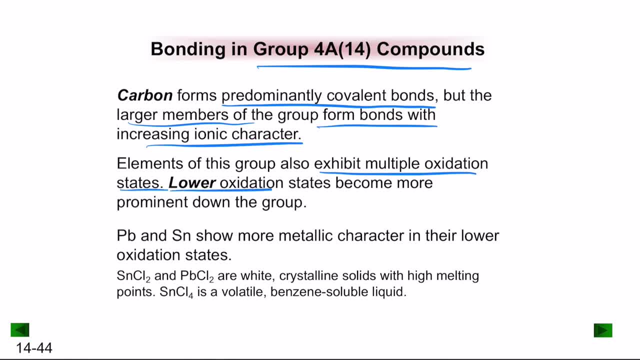 Next elements of this group also exhibit multiple oxidation states. The main reason we discuss because lower oxidation states become more predominant down the group And lead and tin are generally the ones that show more metallic character in their lower oxidation states And you have stannium chloride and lead chloride. 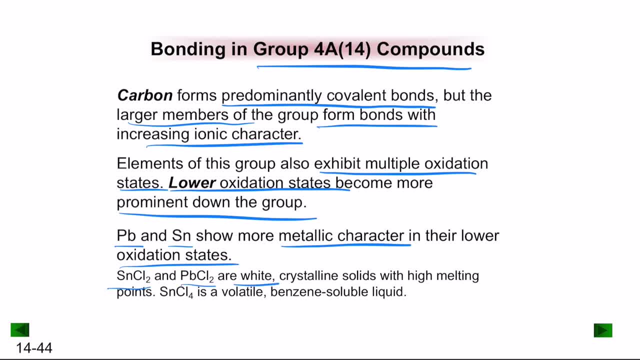 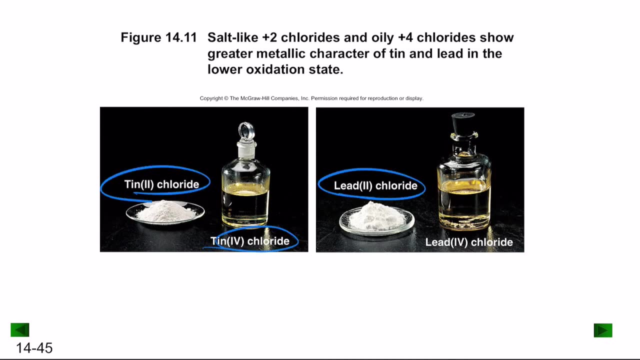 So tin chloride and lead chloride. So these are the elements. Tin and lead chloride generally are white crystalline solids with high melting points, while tin tetrachloride is a volatile, benzene soluble liquid. So this is the difference in terms of the oxidation state, based bonding. 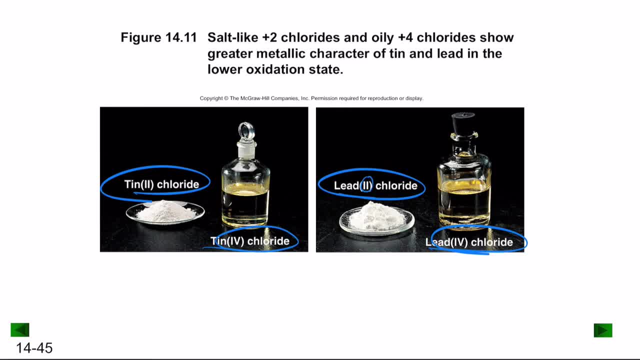 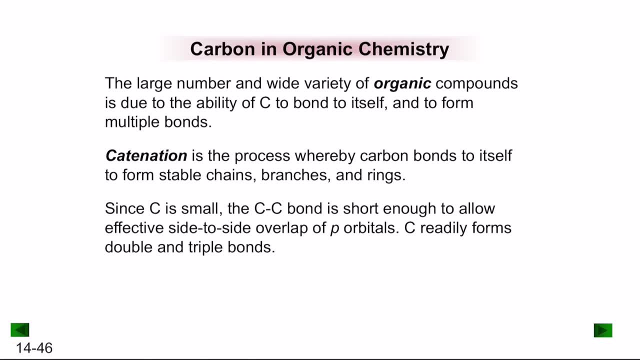 So the type of oxidation state also results in the formation of the type of structure that the material has and the type of phase in which it exists. So another compound that is peculiar in group 4A elements, This is carbon. So the large number and the wide variety of organic compounds is due to the ability of 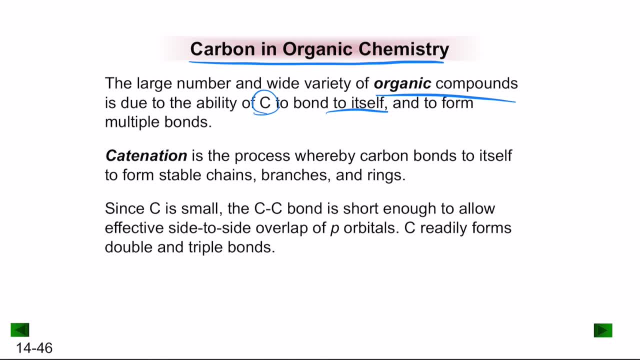 carbon to bond with itself. So this property of an element, where it bonds to itself, is called catenation. So catenation is the process where an element bonds to itself. So this structure, this process, catenation generally involves where carbon bonds with. 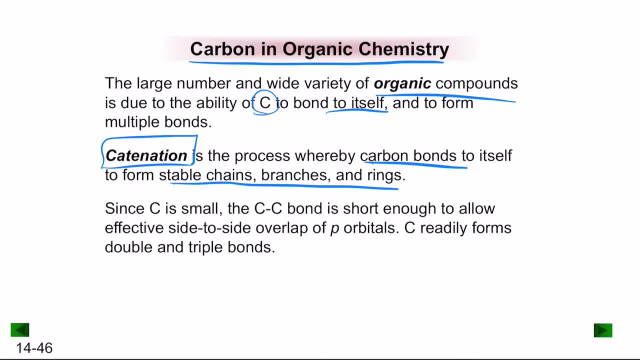 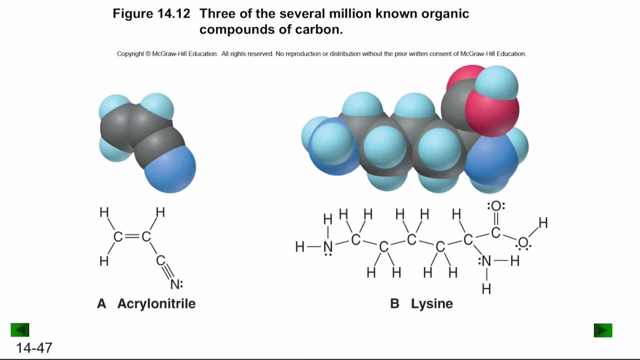 itself to form stable chains, branches and rings, Because carbon is really small. the carbon carbon bond is short enough to allow effective side to side overlap of pion. So this is where you might see acrylonitrile, where the carbons have a double bond and you 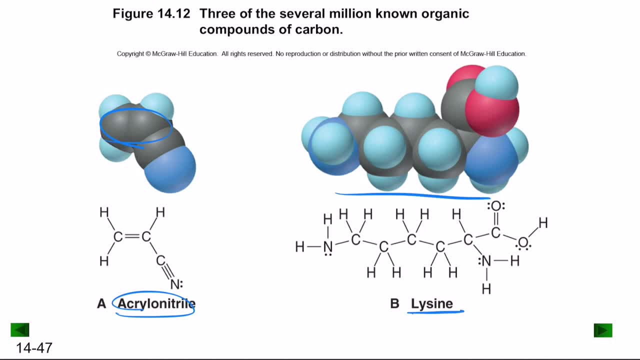 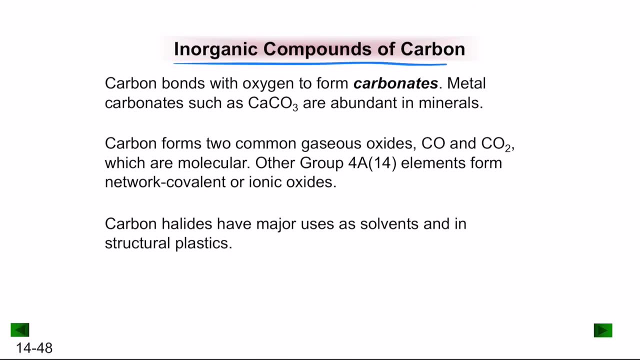 see lysine, which is a continuous carbon structure, So carbon amino acid found in your body. Now, carbon also forms inorganic compounds, So it bonds generally with oxygen to create carbonates, and metal carbonates are generally abundant in minerals. And carbon also forms two common gaseous oxides, carbon monoxide and carbon dioxide, which are 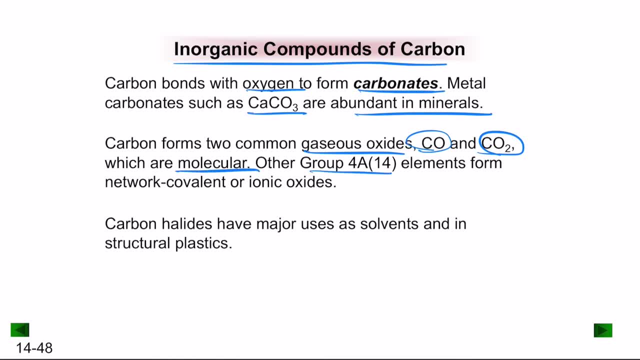 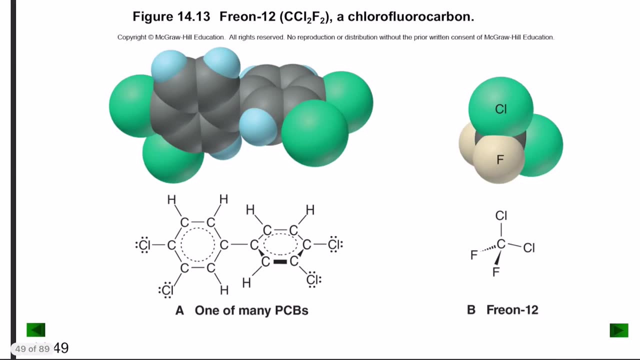 generally molecular and other carbon. other group 4A elements generally form network covalent or ionic oxides. The only one that creates gaseous oxides is carbon. among the group 4A elements Next, carbon halides have major uses as solvents and in structural plastics.